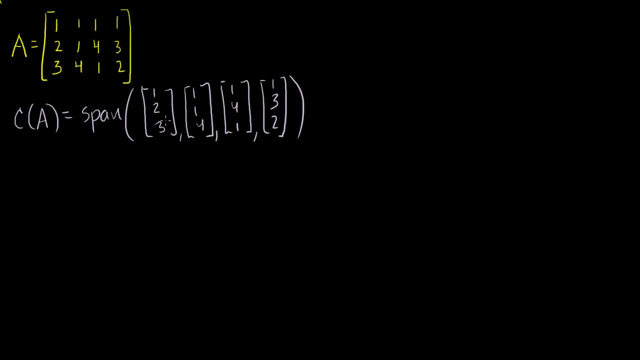 We don't know whether these are linearly independent, But we can figure out if they're linearly independent by looking at the null space of A. Remember, these are linearly independent if the null space of A only contains the 0 vector. 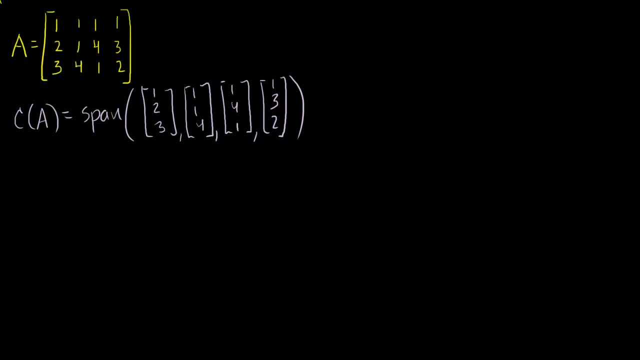 So let's figure out what the null space of A is And remember- we can do a little shortcut here- The null space of A is equal to the null space of the reduced row echelon form, And I showed you that when we first calculated the null space. 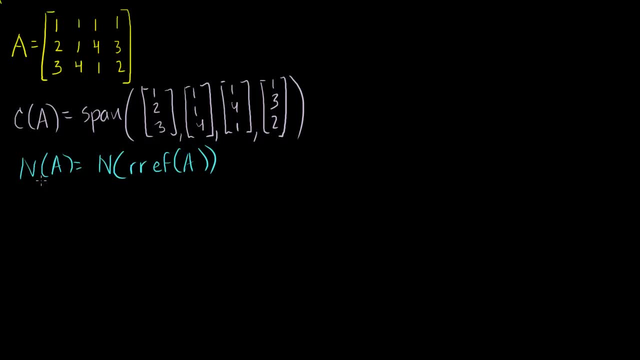 of a vector. Because when you perform these, essentially if you want to solve for the null space of A, you create an augmented matrix And you put the augmented matrix in reduced row echelon form, but the 0's never change. 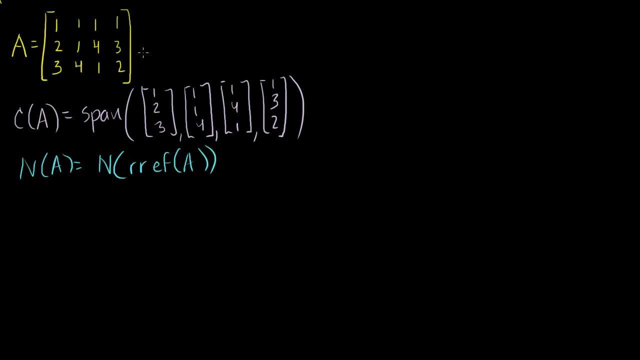 So essentially you're just taking A and putting it in reduced row echelon form. So let's do that. So I'll keep row 1 the same: 1, 1,, 1, 1.. And then let me replace row 2.. 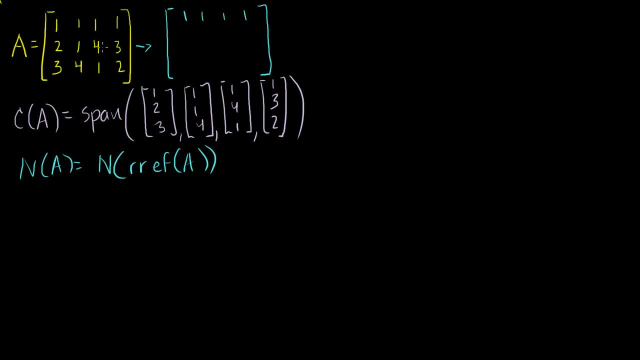 With row 2 minus row 1.. So what do I get? No, actually, I want to 0 this out here. So row 2 minus 2 times row 1.. Actually, even better, Because I eventually want to get a 1 here. 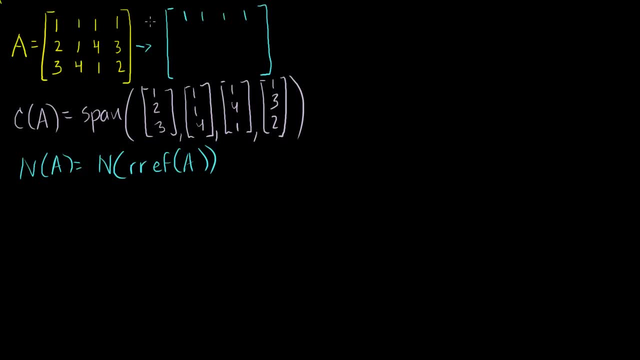 So let me do 2 times row 1 minus row 2.. So let me say 2 times row 1. And I'm going to minus row 2.. So 2 times 1 minus 2 is 0.. Exactly what I wanted there. 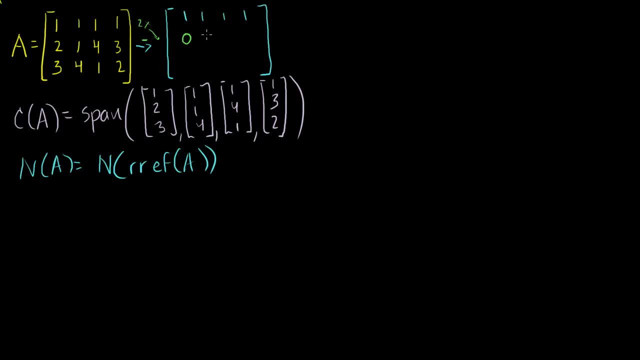 2 times 1 minus 1 is 1.. That's nice to have right there. 2 times 1 minus 4 is minus 2.. 2 times 1 minus 3 is minus 1.. All right, Now let me see if I can 0 out this guy here. 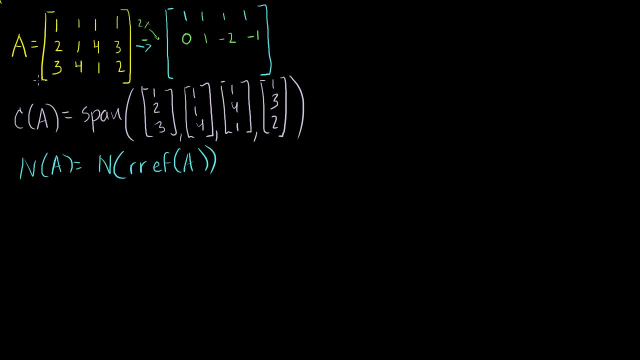 So what can I do? Let's see, I could let me take And I could do it, I could do any combination, Anything that essentially 0s this guy out. But I want to minimize my number of negative numbers. So let me take this third row minus 3 times this first row. 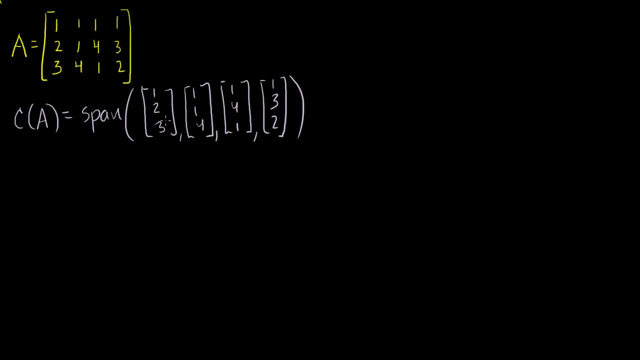 We don't know whether these are linearly independent, But we can figure out if they're linearly independent by looking at the null space of A. Remember, these are linearly independent if the null space of A only contains the 0 vector. 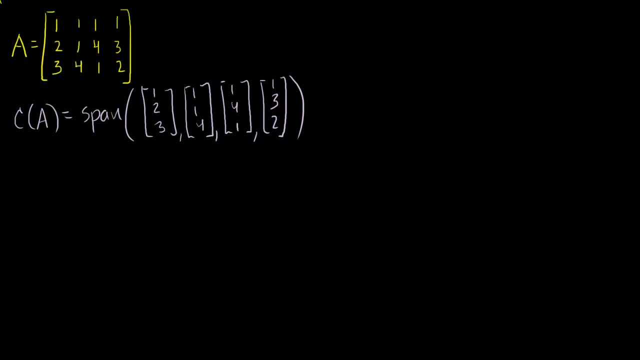 So let's figure out what the null space of A is And remember- we can do a little shortcut here- The null space of A is equal to the null space of the reduced row echelon form, And I showed you that when we first calculated the null space. 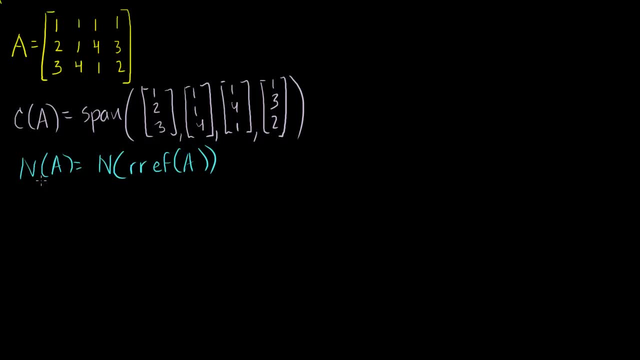 of a vector. Because when you perform these, essentially if you want to solve for the null space of A, you create an augmented matrix And you put the augmented matrix in reduced row echelon form, but the 0's never change. 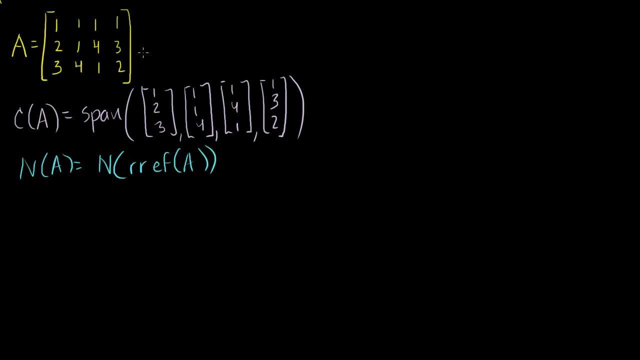 So essentially you're just taking A and putting it in reduced row echelon form. So let's do that. So I'll keep row 1 the same: 1, 1,, 1, 1.. And then let me replace row 2.. 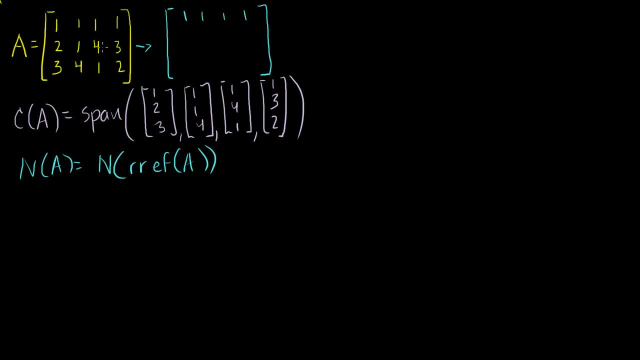 With row 2 minus row 1.. So what do I get? No, actually, I want to 0 this out here. So row 2 minus 2 times row 1.. Actually, even better, Because I eventually want to get a 1 here. 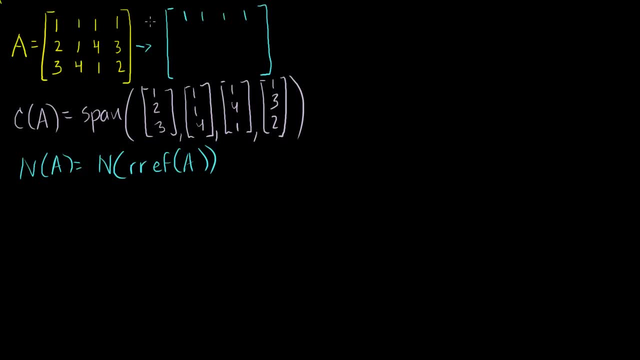 So let me do 2 times row 1 minus row 2.. So let me say 2 times row 1. And I'm going to minus row 2.. So 2 times 1 minus 2 is 0.. Exactly what I wanted there. 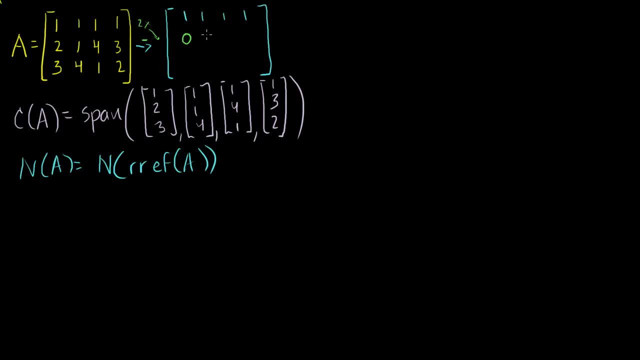 2 times 1 minus 1 is 1.. That's nice to have right there. 2 times 1 minus 4 is minus 2.. 2 times 1 minus 3 is minus 1.. All right, Now let me see if I can 0 out this guy here. 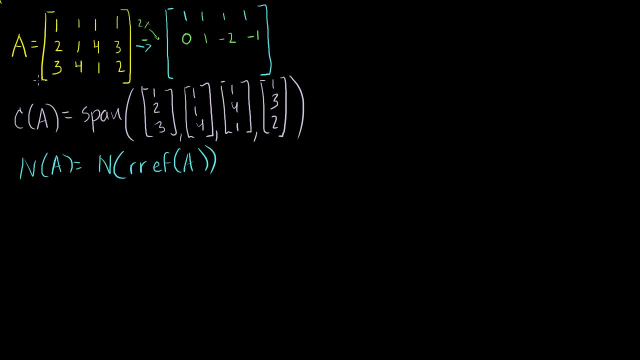 So what can I do? Let's see, I could let me take And I could do it, I could do any combination, Anything that essentially 0s this guy out. But I want to minimize my number of negative numbers. So let me take this third row minus 3 times this first row. 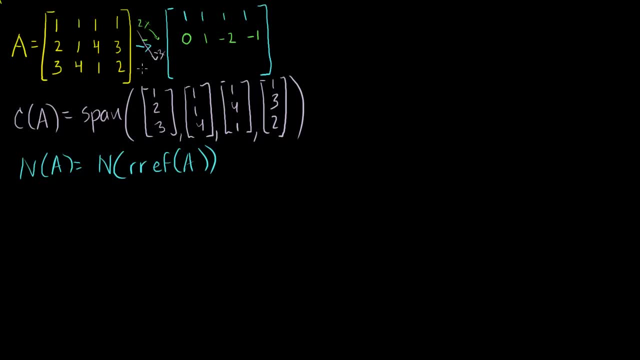 So I'm going to take minus 3 times that first row and add it to this third row. So 3 minus 3 times 1 is 0.. 4 minus 3 times 1.. These are just going to be a bunch of 3s. 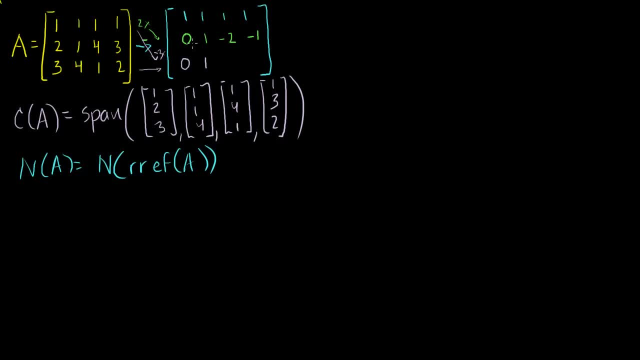 4 minus 3 times 1 is 1.. 1 minus 3 times 1 is 1.. 3 minus 3 times 1 is minus 2.. And 2 minus 3 times 1 is minus 1.. 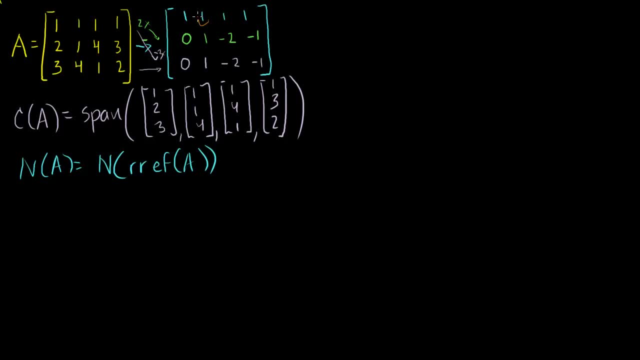 Now, if we want to get this into reduced row echelon form, we need to target that one there and that one there, And what can we do? So let's keep my middle row the same. My middle row is not going to change. 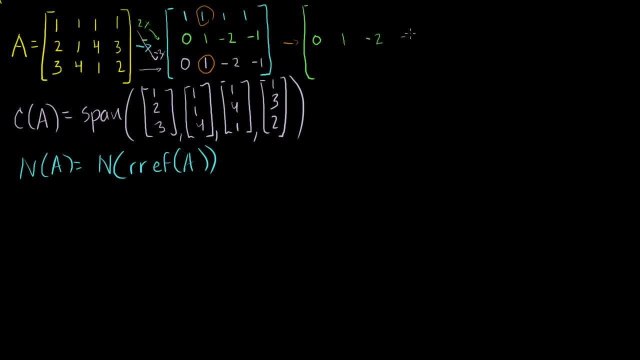 0, 1, minus 2, minus 1.. And to get rid of this one up here, I can just replace my first row with my first row, minus my second row. OK, So I'm going to take my second row, because then this: 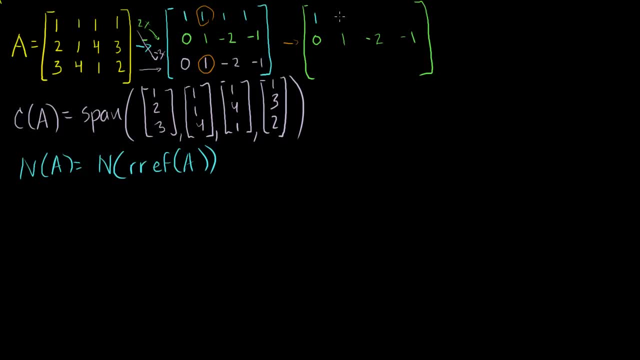 won't change. I'll have: 1 minus 0 is 1.. 1 minus 1 is 0.. That's what we wanted. 1 minus minus 2 is 3, right, That's 1 plus 2.. 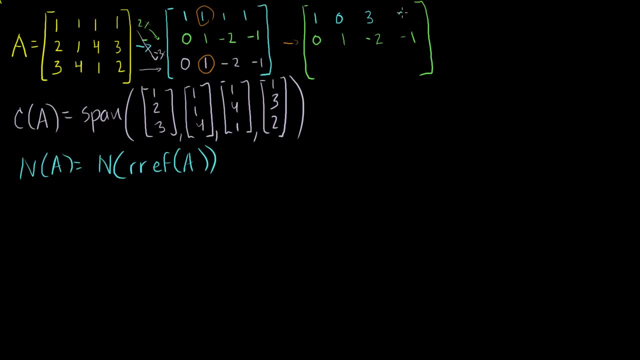 1 minus minus 1, that's 1 plus 1.. That is 2.. Fair enough, Now let me do my third row, The third row. well, let me just add or let me just subtract my. let me replace my third row with my third row. 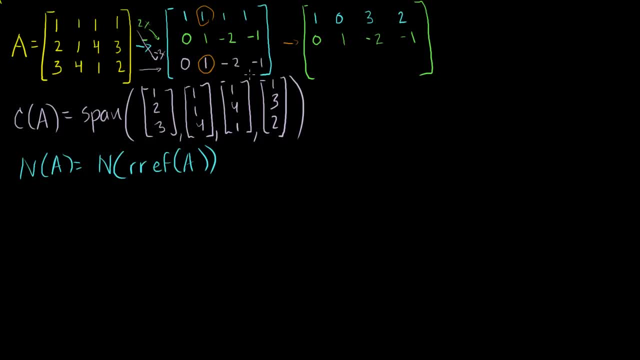 subtracted from my first row, They're obviously the same thing. So if I subtract this row from, if I subtract the third row from the second row, I'm just going to get a bunch of 0's. 0 minus 0 is 0.. 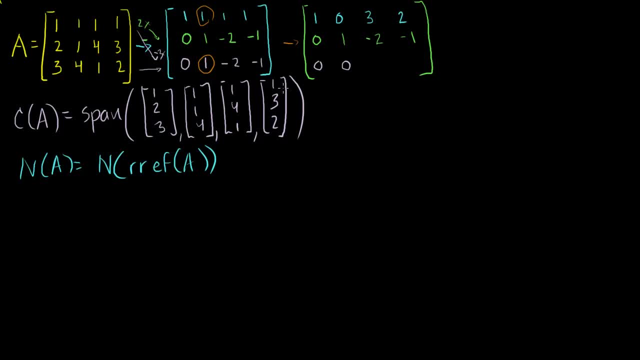 1 minus 1 is 0.. Minus 2 minus minus 2 is 0.. And minus 1 minus minus 1, that's minus 1 plus 1.. That's equal to 0.. And just like that we have it now in reduced row: echelon. 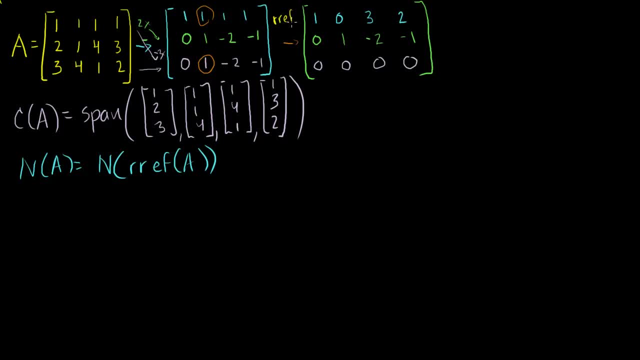 form. So this right here is the reduced row echelon form of a. That straightforward Now the whole reason why we even went through this exercise. we wanted to figure out the null space of a, And we already know that the null space of a is equal to the. 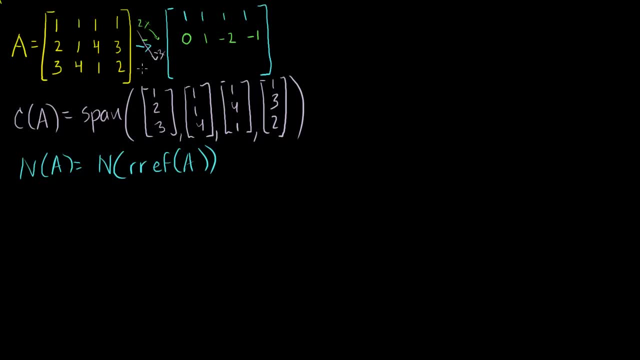 So I'm going to take minus 3 times that first row and add it to this third row. So 3 minus 3 times 1 is 0.. 4 minus 3 times 1.. These are just going to be a bunch of 3s. 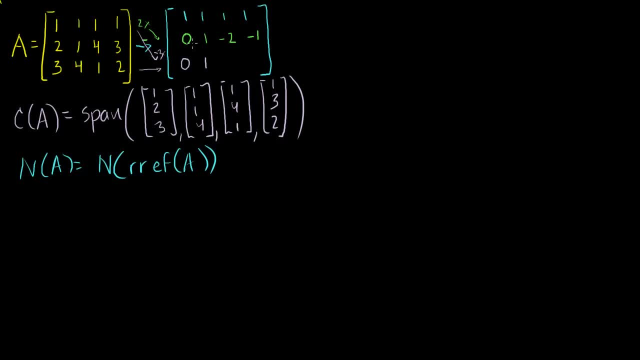 4 minus 3 times 1 is 1.. 1 minus 3 times 1 is 1.. 3 minus 3 times 1 is minus 2.. And 2 minus 3 times 1 is minus 1.. 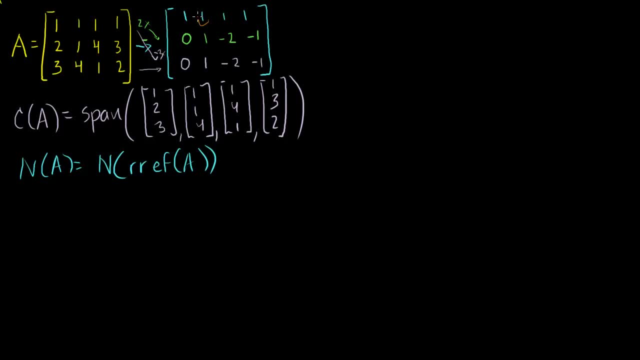 Now, if we want to get this into reduced row echelon form, we need to target that one there and that one there, And what can we do? So let's keep my middle row the same. My middle row is not going to change. 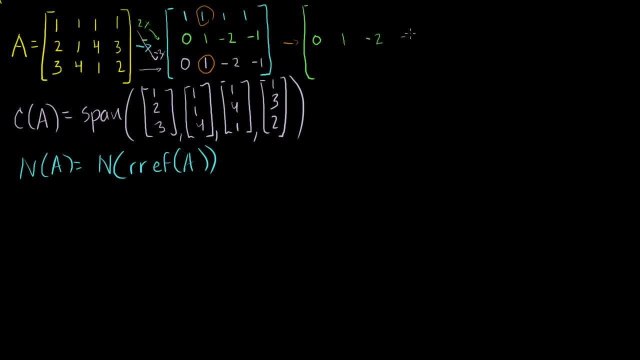 0, 1, minus 2, minus 1.. And to get rid of this one up here, I can just replace my first row with my first row, minus my second row. OK, So I'm going to take my second row, because then this: 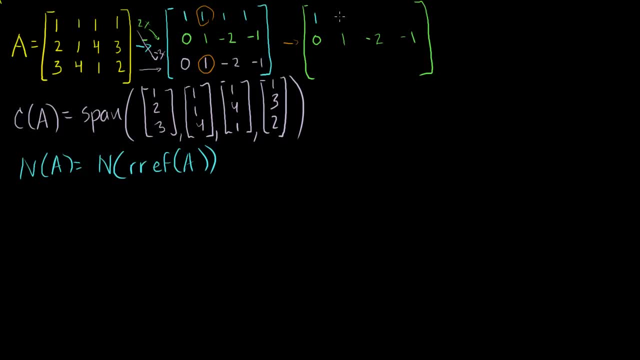 won't change. I'll have: 1 minus 0 is 1.. 1 minus 1 is 0.. That's what we wanted. 1 minus minus 2 is 3, right, That's 1 plus 2.. 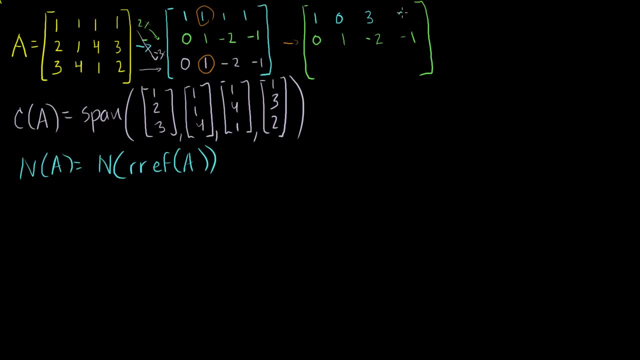 1 minus minus 1, that's 1 plus 1.. That is 2.. Fair enough, Now let me do my third row, The third row. well, let me just add or let me just subtract my. let me replace my third row with my third row. 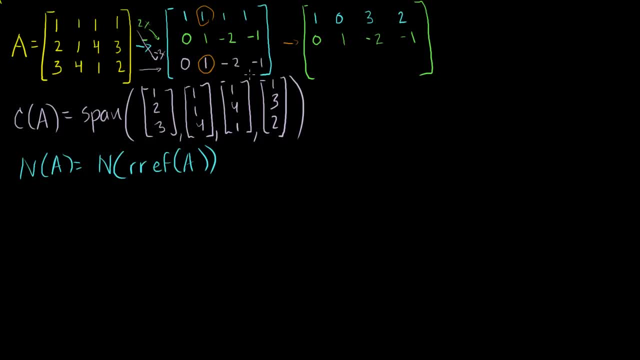 subtracted from my first row, They're obviously the same thing. So if I subtract this row from, if I subtract the third row from the second row, I'm just going to get a bunch of 0's. 0 minus 0 is 0.. 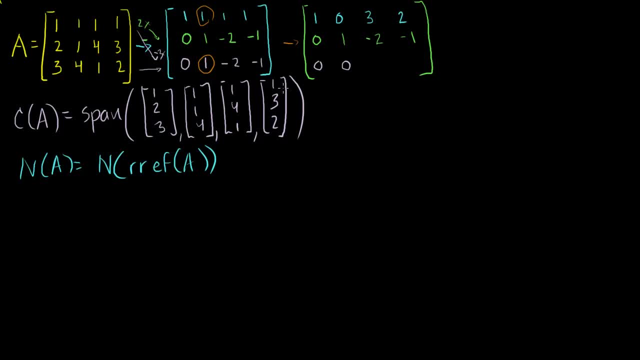 1 minus 1 is 0.. Minus 2 minus minus 2 is 0.. And minus 1 minus minus 1, that's minus 1 plus 1.. That's equal to 0.. And just like that we have it now in reduced row: echelon. 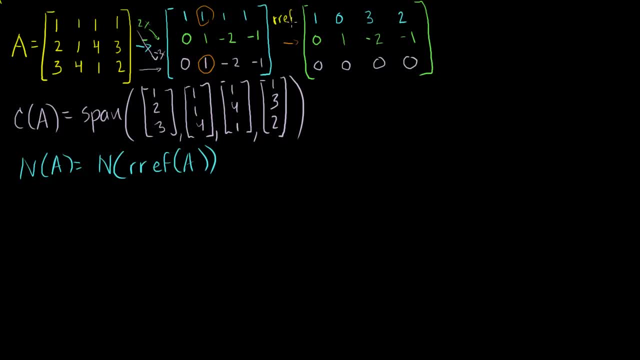 form. So this right here is the reduced row echelon form of a. That straightforward. Now. the whole reason why we even went through this exercise is we wanted to figure out the null space of a, and we already know that the null space of a is equal to the null. 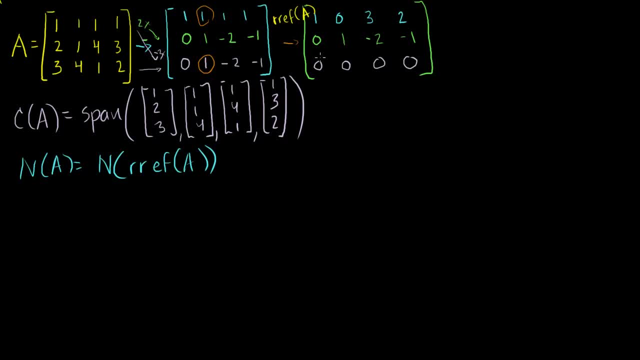 null space of the reduced row echelon form of a. So if this the reduce row echelon form of a, let's figure out its null space. So the null space is a set of all vectors and r4, because we have 4 columns here. 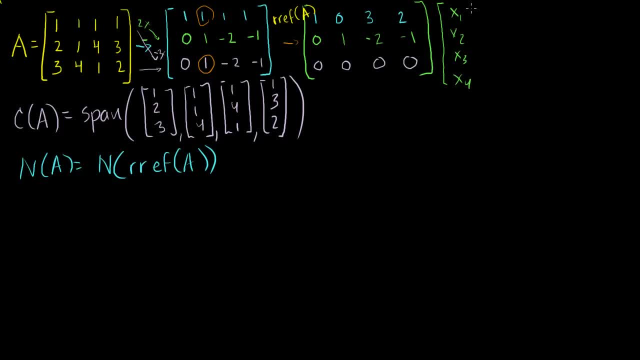 1,, 2,, 3, 4.. The null space is the set of all vectors that satisfy this equation. We're going to have three 0's right here. That's the 0 vector in R3, because we have three rows. 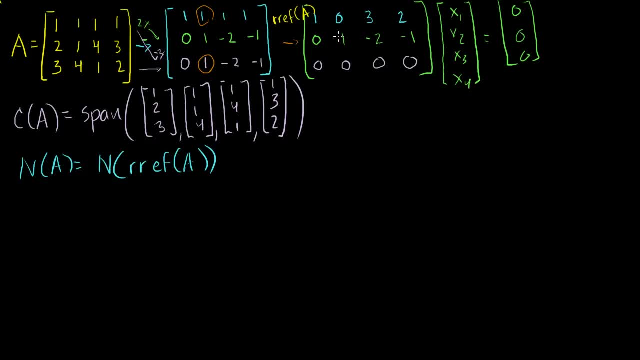 right there and you can figure it out. This times this has to equal that 0.. That dotted with that, essentially, is going to equal that 0. That dotted with that is equal to that 0.. I say essentially because I didn't define a row vector. 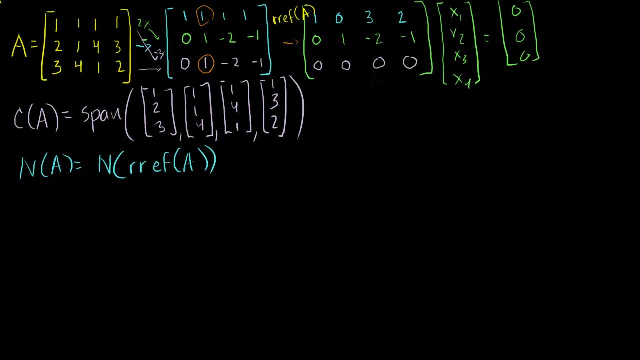 dot a column vector. I've only defined column vectors dotted with other column vectors, but we've covered that in a previous video where you could just say: this is a transpose of a column vector, So let's just take this and write a system of 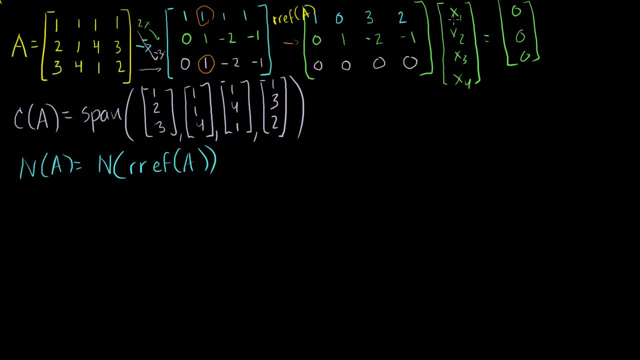 equations with this. So we get 1 times x1.. So this times this is going to be equal to that 0. So 1 times x1, that is x1, plus 0 times x2.. Let me just write that out. 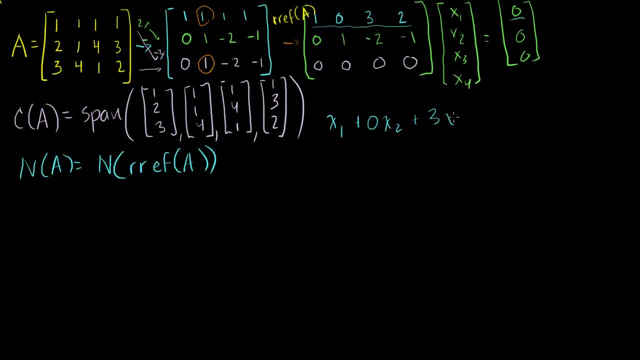 Plus 0 times x2, plus 3 times x3, plus 2 times x4 is equal to that 0.. Right, 0 is equal to 0.. And then in yellow right here I have 0 times x1, plus 1 times. 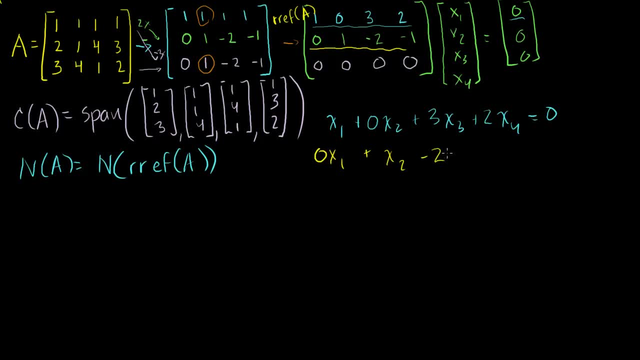 x2, minus 2 times x3, minus x4 is equal to 0. And then- this gives me no information- 0's times all of this is equal to 0. So it just turns into 0 equals 0. 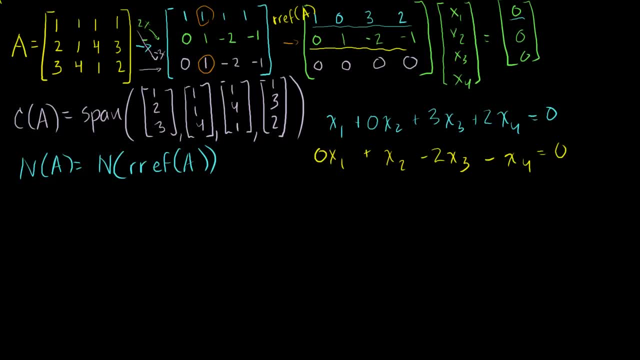 So let's see if we can solve for our pivot entries or our pivot variables. What are our pivot entries? This is a pivot entry. That's a pivot entry. That's what reduced row echelon form is all about getting these entries that are 1, and they're the only non-zero term. 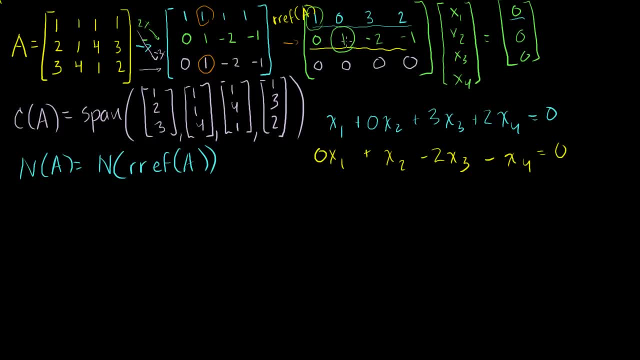 in their respective columns and that every pivot entry is to the right of a pivot entry above it. And then the columns that don't have pivot entries. these columns represent the free variables. So this column has no pivot entry And so when you take the dot product, this column turned. 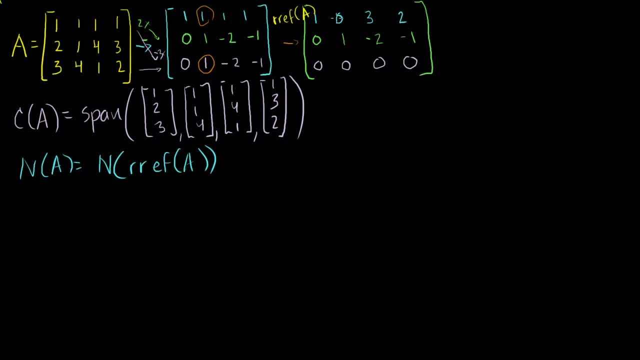 space of the reduced row echelon form of a. So if this is the reduced row echelon form of a, let's figure out its null space. So the null space is the set of all vectors in R4, because we have four columns here. 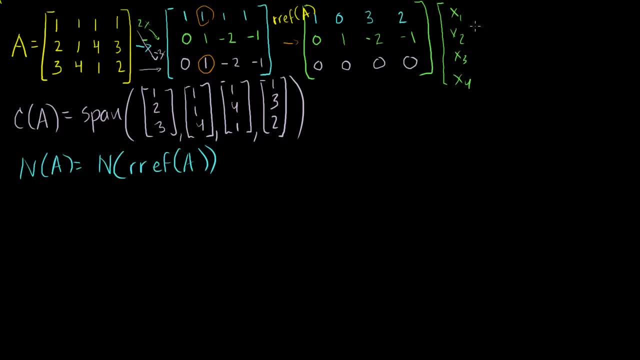 1,, 2,, 3, 4.. The null space is the set of all vectors. OK, OK, that satisfy this equation. We're going to have three 0's right here. That's the 0 vector in R3, because we have three rows. 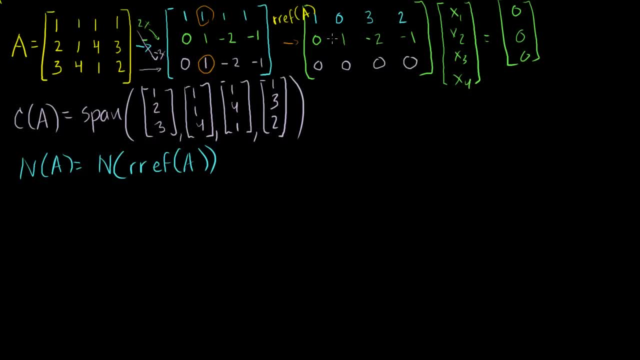 right there and you can figure it out. This times this has to equal that 0.. That dotted with that, essentially, is going to equal that 0. That dotted with that is equal to that 0.. I say essentially because I didn't define a row vector. 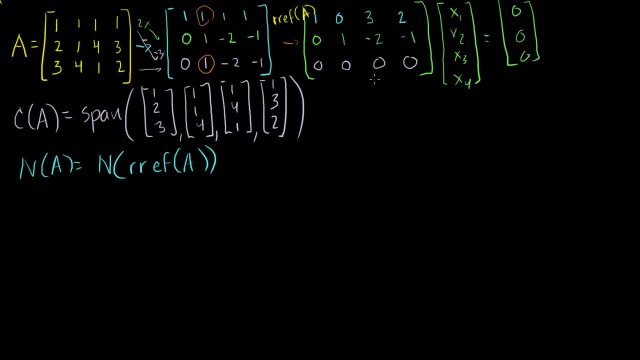 dot a column vector. I've only defined column vectors dotted with other column vectors, but we've covered that in a previous video, where you could just say: this is a transpose of a column vector. Let's just take this and write a system of 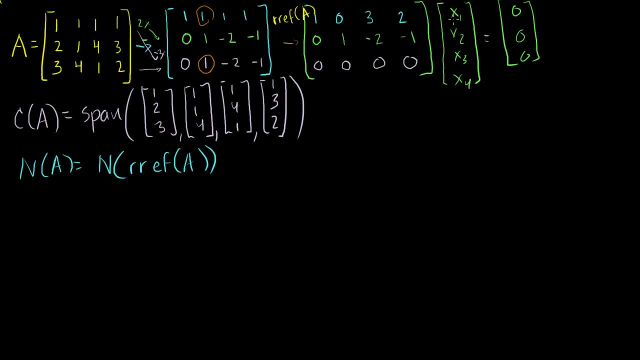 equations. with this We get 1 times x1. This times this is going to be equal to that 0.. 1 times x1, that is x1, plus 0 times x2.. Let me just write that out: Plus 0 times x2, plus 3 times x3, plus 2 times x4 is equal. 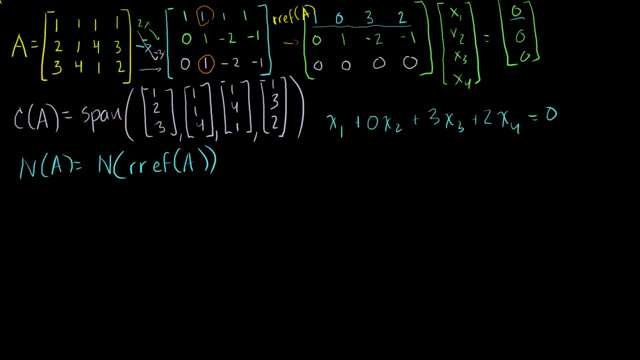 to that 0.. That's the transpose of a column vector: 0 is equal to 0.. And then in yellow right here I have 0 times x1, plus 1 times x2, minus 2 times x3, minus x4 is equal to 0.. 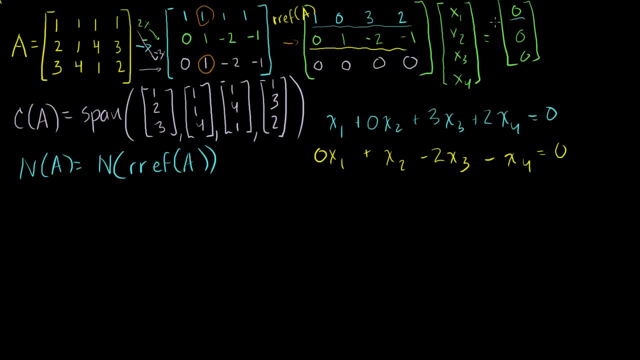 And then this gives me no information: 0's times. all of this is equal to 0. So it just turns into 0 equals 0. So let's see if we can solve for our pivot entries or our pivot variables. What are our pivot entries? 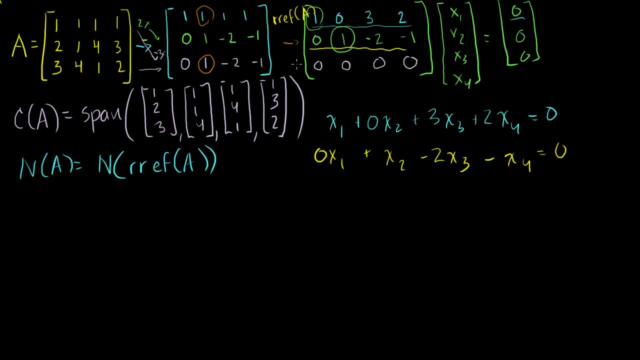 This is a pivot entry. That's a pivot entry. That's what reduced row echelon form is all about: getting these entries that are 1, and they're the only non-zero term in their respective columns, and that every pivot entry is. 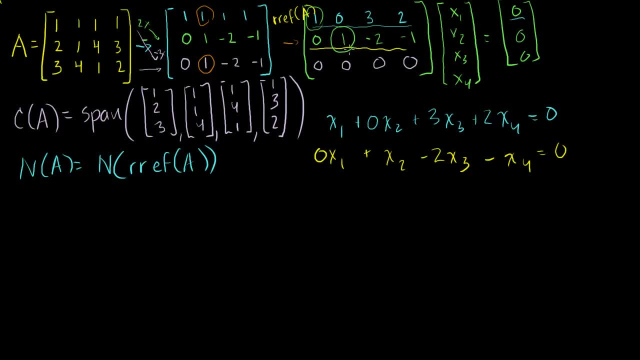 to the right of a pivot entry above it, And then the columns that don't have pivot entries. these columns represent the free variables, So this column has no pivot entry And so when you take the dot product, this column turned into this column in our system. 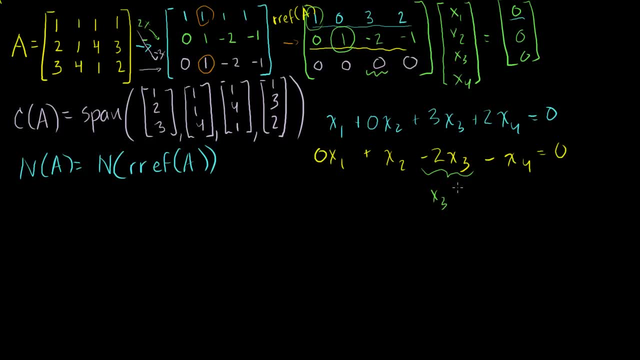 It's a system of equations, so we know that x3 is a free variable. x3 is free. We can set it equal to anything. Likewise, x4 is free is a free variable. x1 and x2 are pivot variables because their corresponding 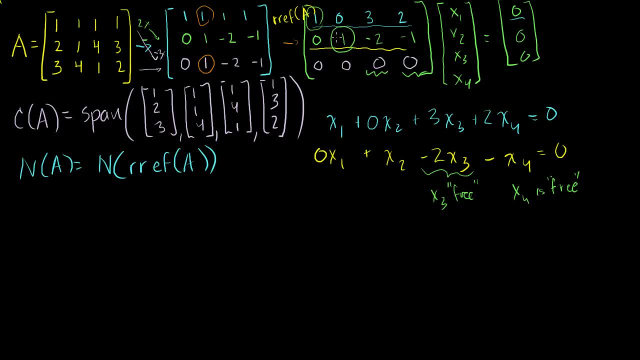 columns in our reduced row echelon form have pivot entries in them. Fair enough, So let's see if we can simplify this into a form we know And we've seen this before. So if I solve for x1. This 0 I can ignore. 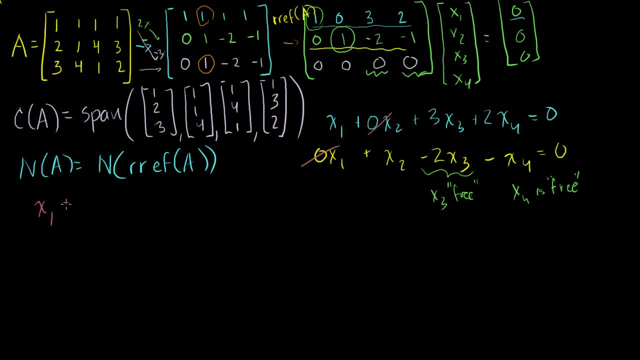 That 0 I can ignore. I could say that x1 is equal to minus 3x3, minus 2x4.. I just subtracted these two from both sides of the equation and I can say that x2 is equal to 2x3 plus x4. 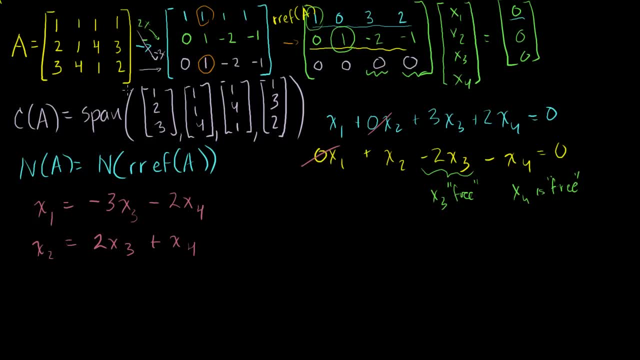 And if we want to write our solution set now. so if I wanted to find the number, I can find the null space of a. So the null space of a, which is the same thing as the null space of the reduced row, echelon form of a is equal to. 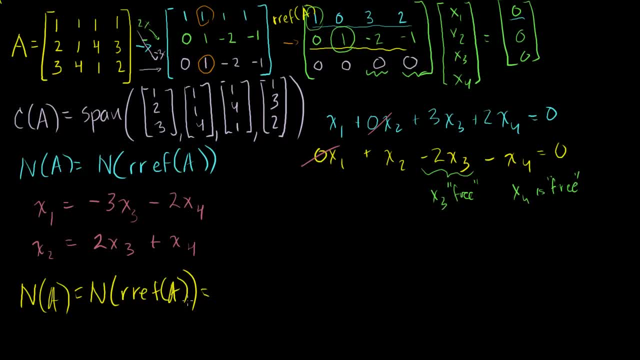 all of the vectors. Let me do a new color, Maybe I'll do blue. It's equal to all of the vectors x1, x2, x3, x4 that are equal to. So what are they going to be equal to? x1 has to be equal. 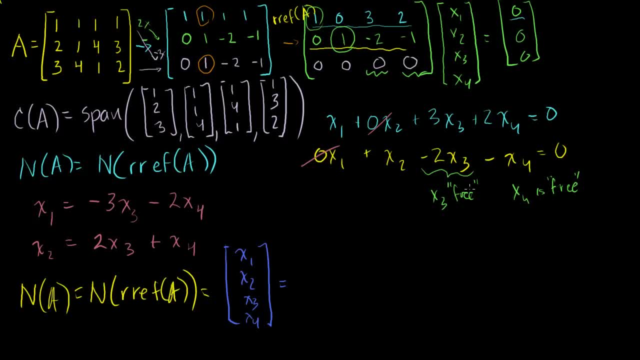 to minus 3x3x4.. x3x4.. So just to be clear, these are free variables because I can set these to be anything, And these are pivot variables because I can't just set them to anything. When I determine what my x3's and my x4's are, they determine: 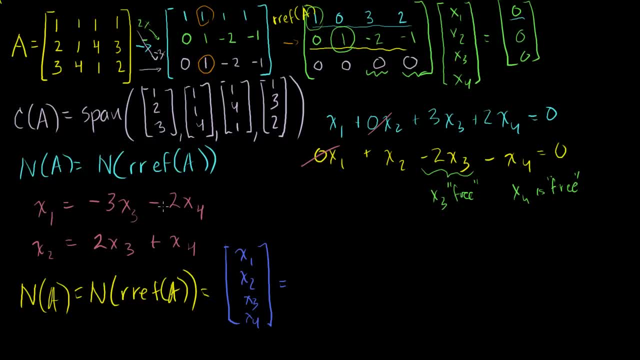 what my x1's and my x2's have to be. So these are pivoted variables, These are free variables. I can make this guy pi and I can make this guy minus 2.. We can set them to anything. So x1 is equal to. let's see, let me write it this way. 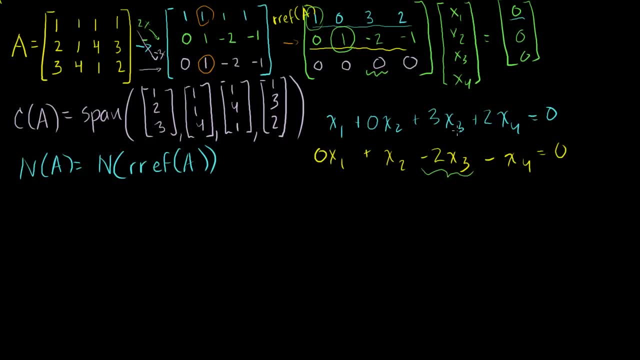 into this column. in our system It's a system of equations, so we know that x3 is a free variable. x3 is free. We can set it equal to anything. Likewise, x4 is free. x1 and x2 are pivot variables because their corresponding 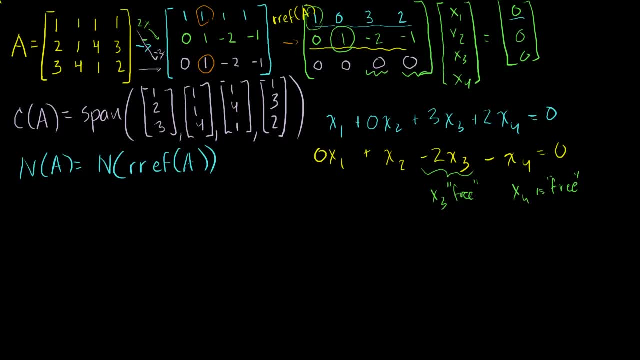 columns in our reduced row echelon form have pivot entries in them. Fair enough. So let's see if we can simplify this into a form we know And we've seen this before. So if I solve for x1, this 0, I can ignore, that 0 I can. 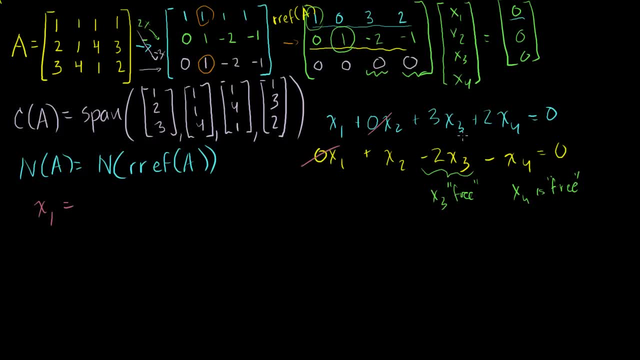 ignore. I could say that x1 is equal to minus 3x3 minus 2x4.. Right, I just subtracted these two from both sides of the equation and I can say that x2 is equal to 2x3 plus x4. 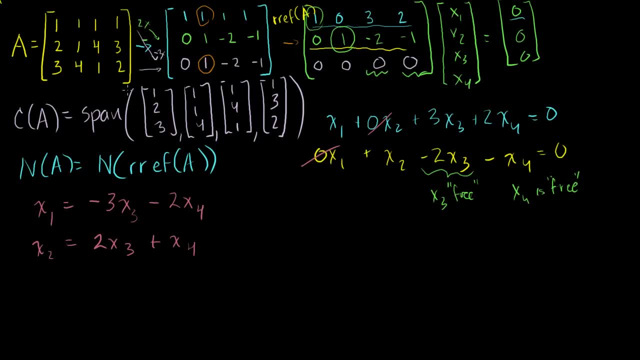 And if we want to write our solution set now. so if I wanted to find the null space of A, which is the same thing as the null space of the reduced row, echelon form of A is equal to all of the vectors. 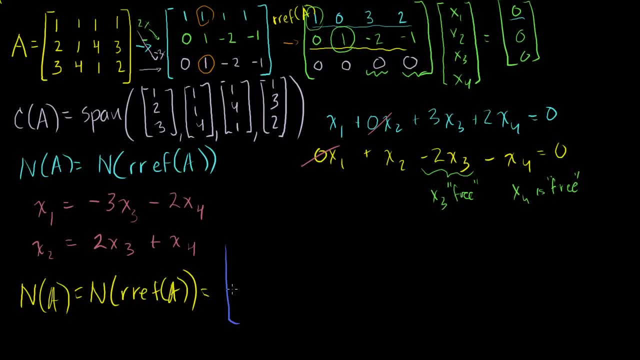 Let me do a new color. Maybe I'll do blue. It's equal to all of the vectors x1, x2, x3, x4 that are equal to. so what are they going to be equal to? x1 has to be equal to minus 3x3, minus 2x4.. 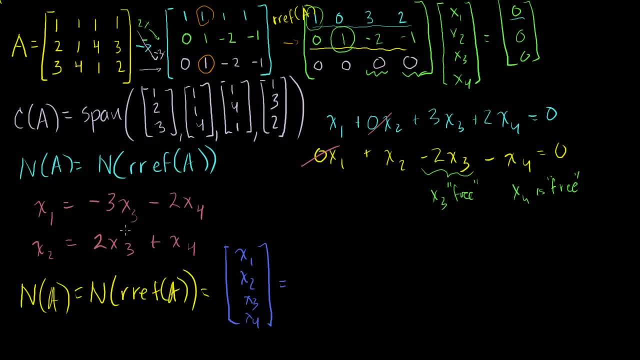 So, just to be clear, these are free variables because I can set these to be anything, And these are pivot variables because I can't just set them to anything. When I determine what my x3's and my x4's are, they determine: 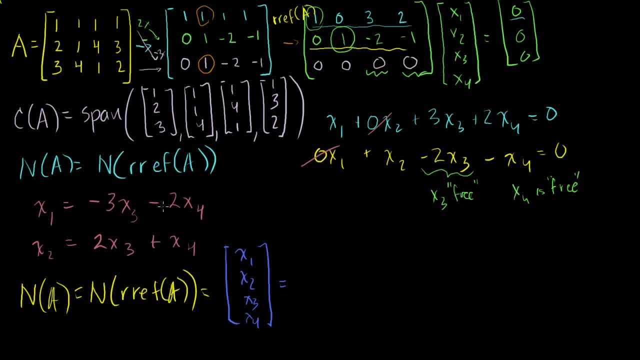 what my x1's and my x2's have to be. So these are pivoted variables, These are free variables. I can make this guy pi and I can make this guy minus 2.. We can set them to anything. So x1 is equal to. let's see, let me write it this way. 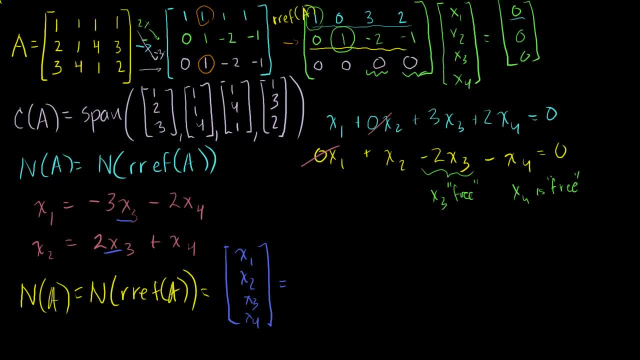 They're equal to x3.. Let me do it in a different color. Do x3 like this, So it's equal to x3 times some vector plus x4 times some other vector. So any solution set in my null space is going to be a linear. 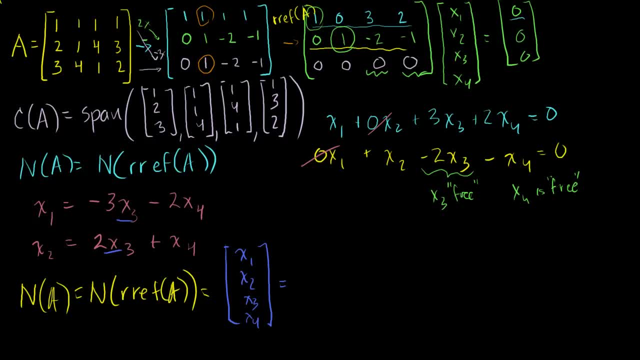 They're equal to x3.. Let me do it in a different color. Do x3 like this, So it's equal to x3 times some vector plus x4 times some other vector. So any solution set in my null space is going to be a linear. 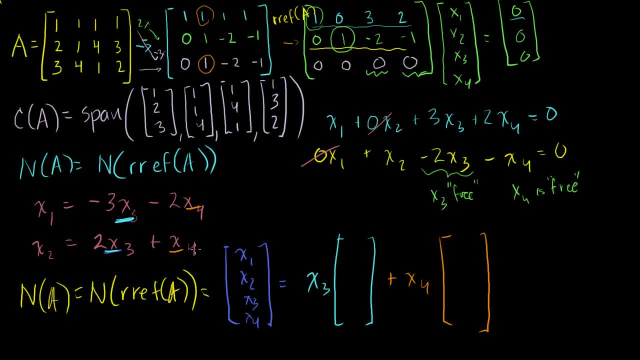 combination of these two vectors, And we can figure out what these two vectors are just from these two constraints right here. So let me do it in a neutral color. x1 is equal to x2.. So x1 is equal to x2.. 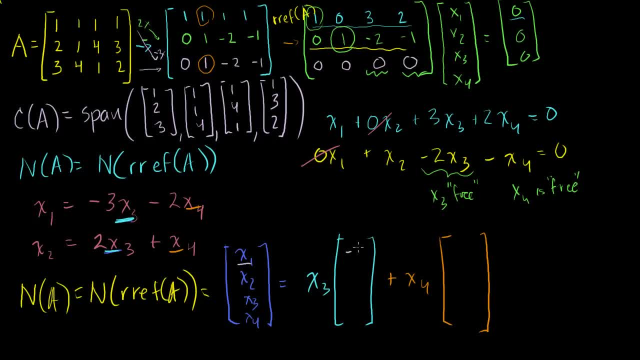 So x2 is equal to minus 3 times x3.. So minus 3 times x3, minus 2 times x4. Straightforward enough: x2 is equal to 2 times x3 plus x4.. What's x3 equal to? 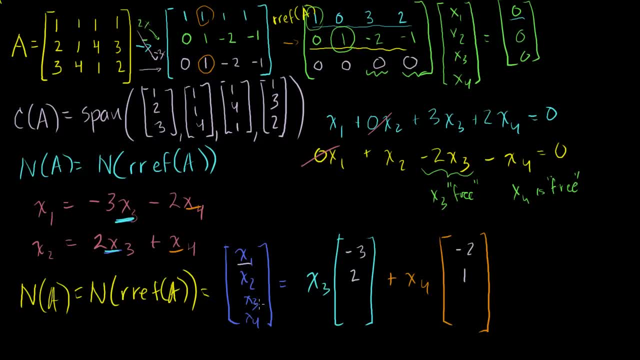 Well, x3 is equal to itself. Whatever we set x3 equal to, that's going to be x3. So x3 is going to be 1 times x3 plus 0 times x4. It's not going to have any x4 in it. 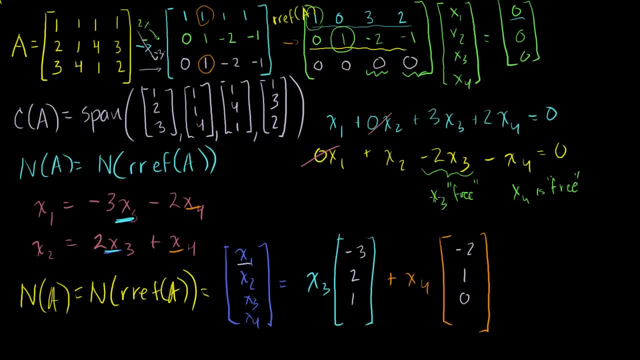 x3 is going to be kind of an independent variable where it's going to be free. We can set it to whatever it is. So we set it and then that's going to be our x3 in our solution. set x4 is not going to have any x3 in it. 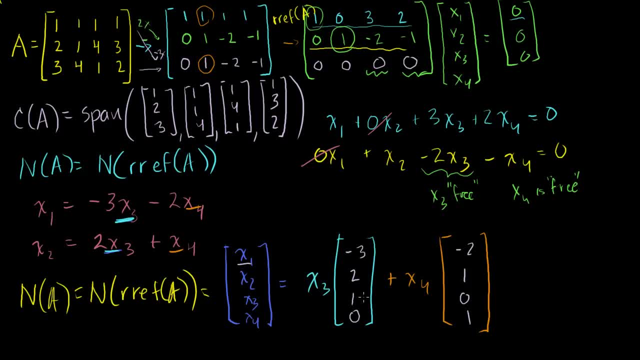 It's just going to be 1 times x4.. And so our null space is essentially all of the linear combinations of these two vectors. right, This can be any real number. This is just any real number, And x4 is just any member of the real space. 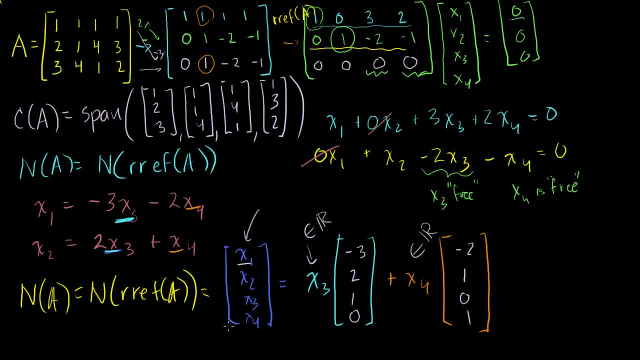 So all of these, the set of all of the valid solutions to ax, is equal to 0.. Where did I write that? Did I even write that? No, I haven't even written that anywhere. The set of all ax is equal to 0, where this is my x: it. 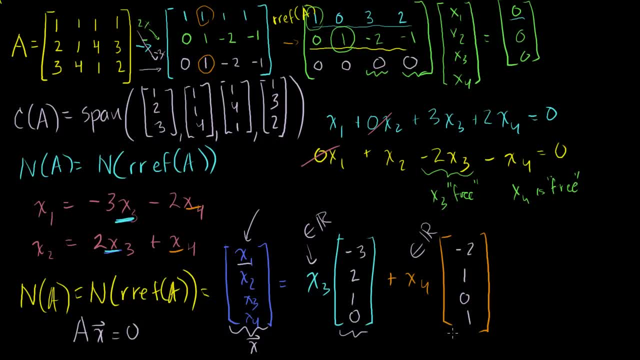 equals all of the linear combinations of this vector and that vector right there, And we know what all of the linear combinations mean. It means my null space is equal to the span of these two guys, the span of minus 3, 2, 1, 0. 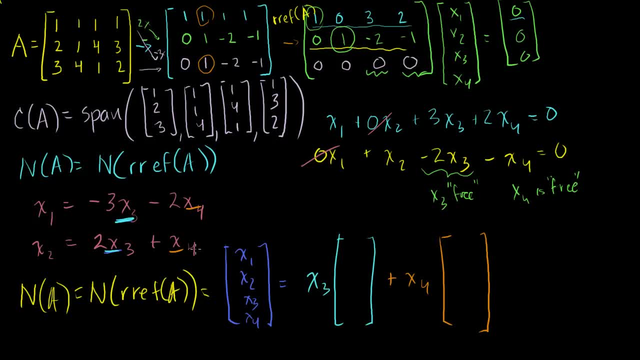 combination of these two vectors, And we can figure out what these two vectors are just from these two constraints right here. So let me do it in a neutral color. x1 is equal to minus 3 times x3.. So minus 3 times x3, minus 2 times x4. 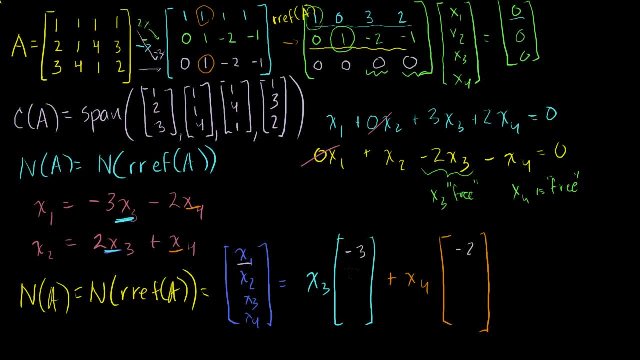 Straightforward enough: x2 is equal to 2 times x3 plus x4.. What's x3 equal to? Well, x3 is equal to itself. Whatever we set x3 equal to, that's going to be x3.. So x3 is going to be 1 times x3 plus 0 times x4. 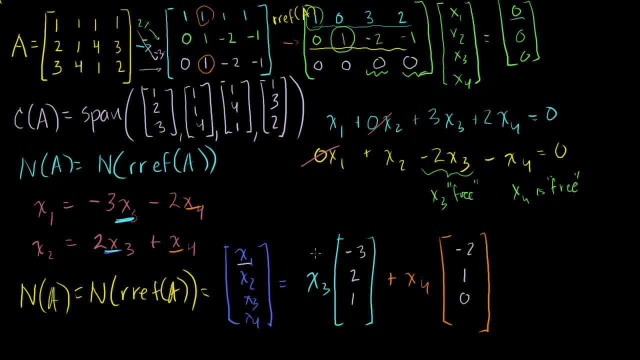 It's not going to have any x4 in it. x3 is going to be kind of an independent vector. It's going to be independent vector. It's going to be independent vector. It's going to be independent variable where it's going to. 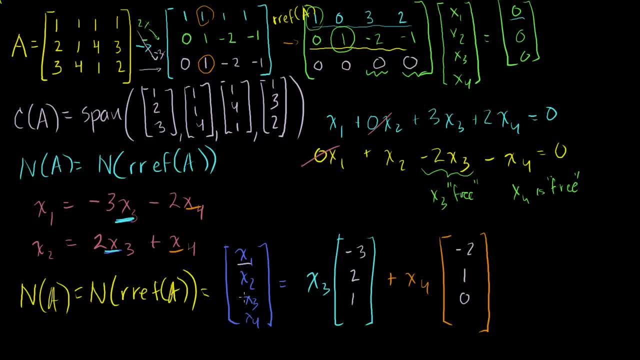 be free, We can set it to whatever it is. So we set it and then that's going to be our x3 in our solution. set x4 is not going to have any x3 in it, It's just going to be 1 times x4. 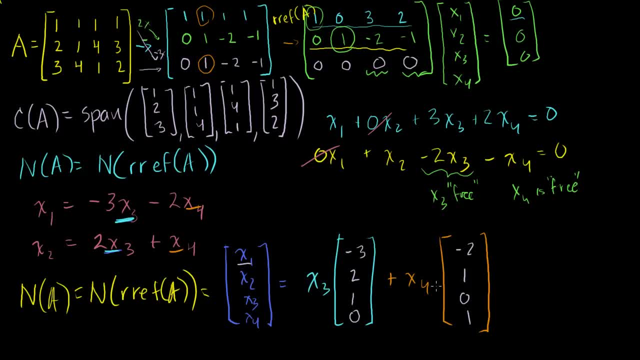 And so our null space is essentially all of the linear combinations of these two vectors. right, This can be any real number, This is just any real number, And x4 is just any member of the real space. So all of these, the set of all of the valid solutions to 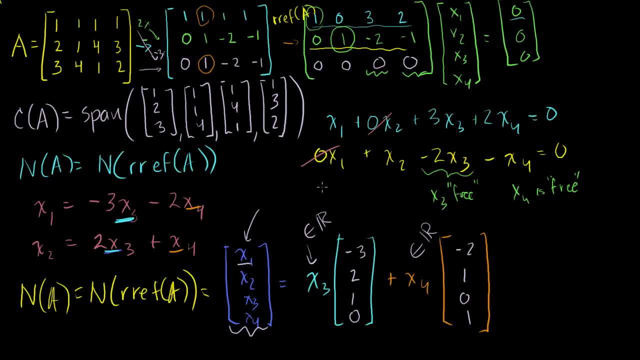 ax is equal to 0.. Where did I write that? Did I even write that down? No, I haven't even written that anywhere. The set of all ax is equal to 0, where this is my x, it equals all of the linear combinations of this vector. 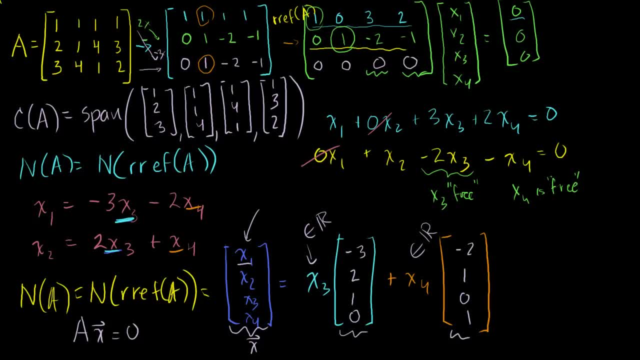 and that vector right there, And we know what all of the linear combinations mean. It means: so my null space- let me write it this way- is equal to the span of these two guys, The span of minus 3, 2, 1, 0. 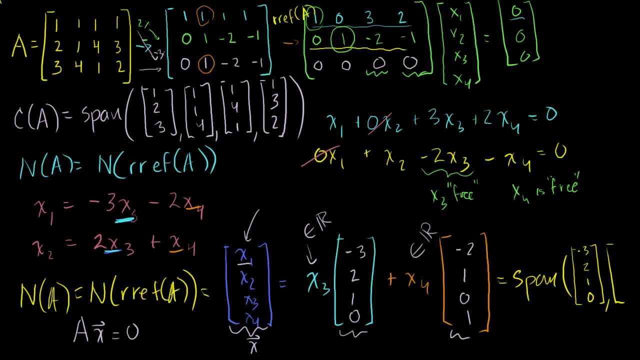 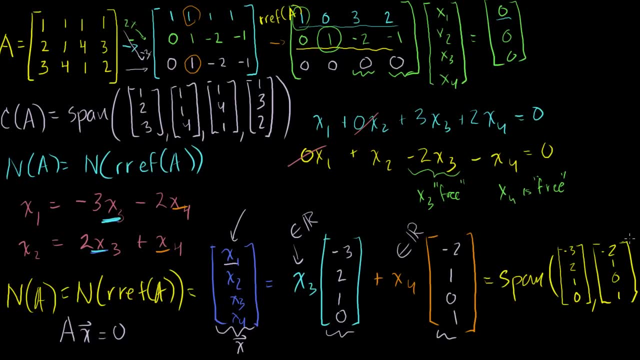 And let me scroll over a little bit- And minus 2,, 1,, 0,, 1.. Now let me ask you a question: Are the columns in A? are they a linearly independent set? Let me write that down. 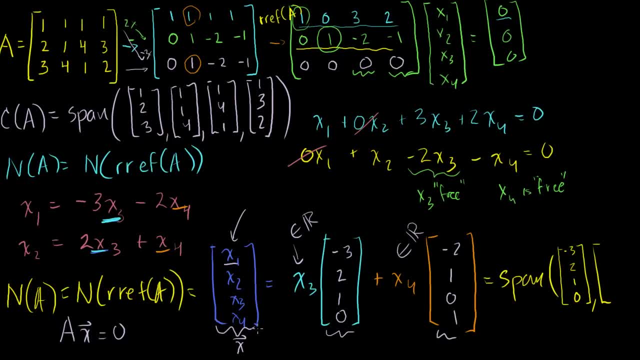 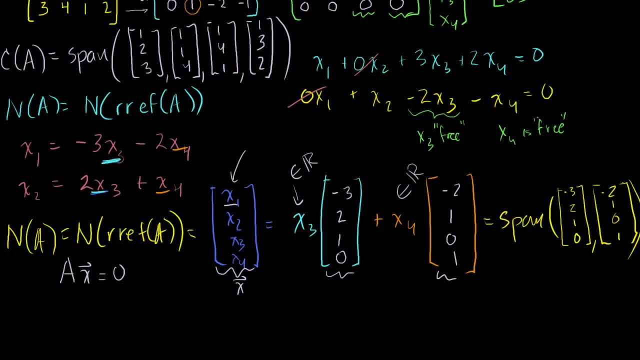 And let me scroll over a little bit- And minus 2,, 1,, 0,, 1.. Now let me ask you a question: Are the columns in A? are they a linearly independent set? Let me write that down. 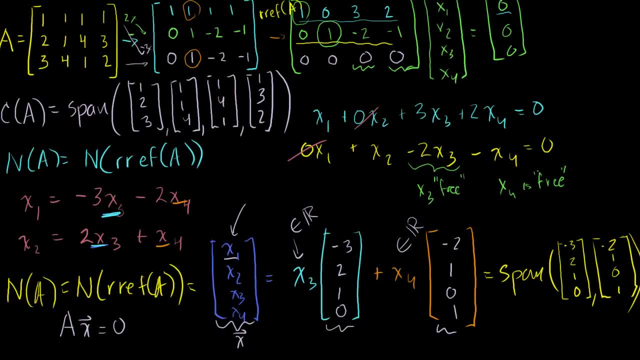 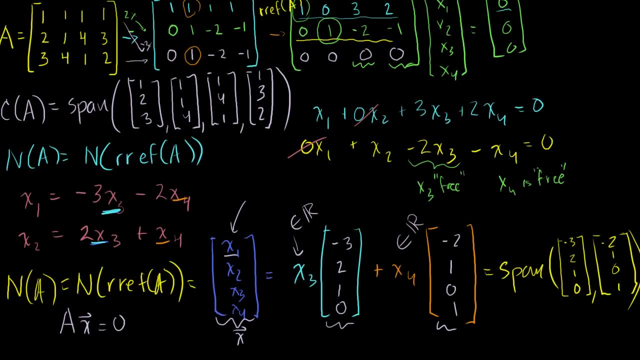 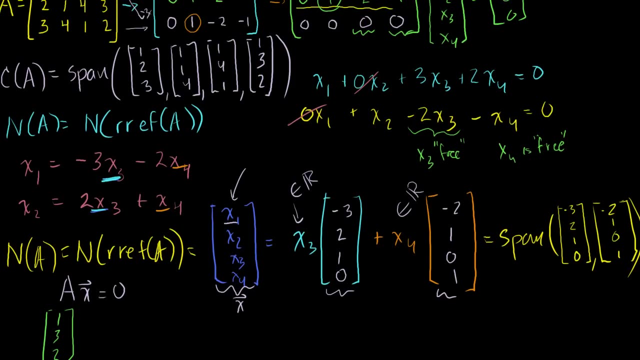 So if we write these vectors right there, these are the vectors, the column vectors of A. So let me write that down. So are the column vectors of A. so what were they? Let's see: 1,, 1,, 3,, 2, I don't remember them. 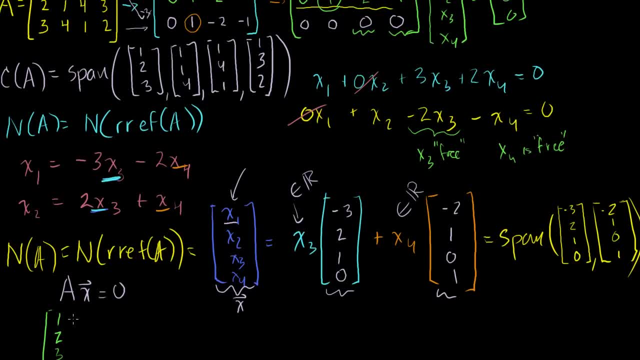 No, it's 1, 2, 3.. 1, 2, 3,, 1, 1, 4,, 1, 4, 1, and 1, 3, 2.. So this is just the. 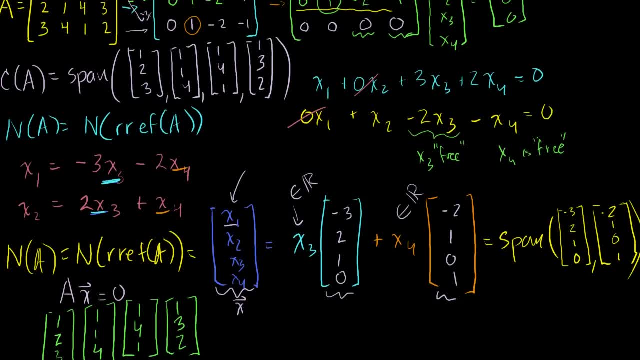 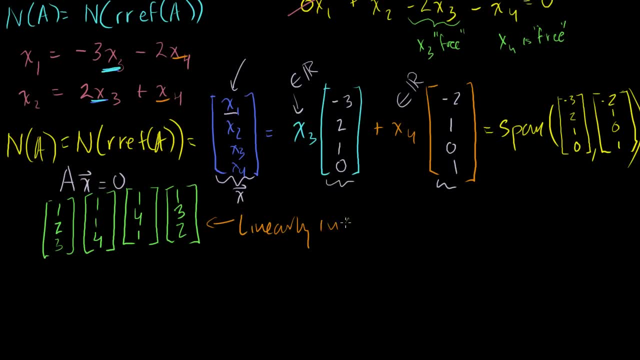 column. vectors of A. I could just write A as just this much of columns. But my question is: is this a linearly independent set? Linearly independent? And here you might immediately start thinking: well, when we said that something is. 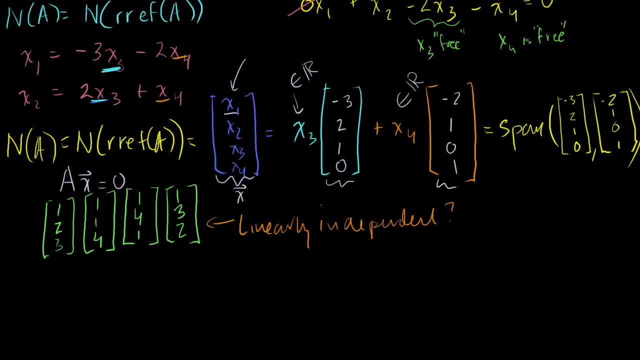 linearly independent. So linearly independence. let me just write it like this: Linear independence implies that there's only one solution. We saw this, I think, two videos ago. That there's only one solution to Ax is equal to 0.. 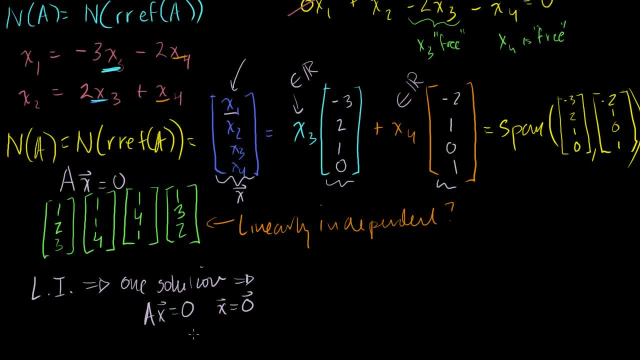 And that is the 0 solution, That x is equal to the 0 vector. Or another way to say that is that the null space of my matrix A is equal to just the 0 vector. That's what linear independence implies, And it goes both ways. 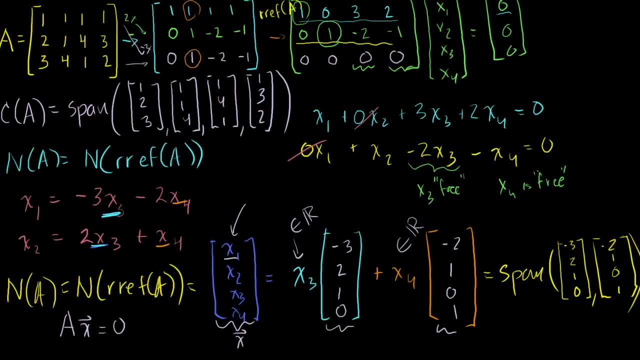 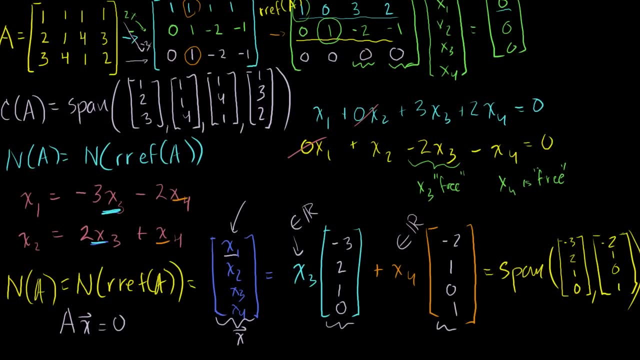 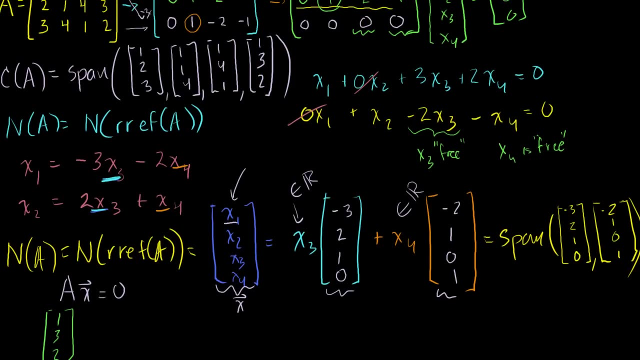 So if we write these vectors right there, These are the vectors, the column vectors of A. So let me write that down. So are the column vectors of A. so what were they? Let's see: 1,, 1,, 3,, 2, I don't remember them. 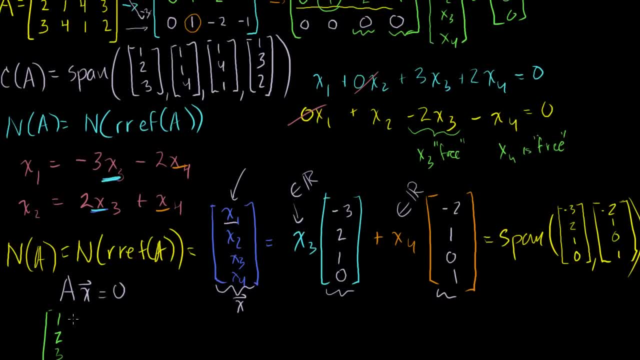 No, it's 1, 2, 3.. 1, 2, 3,, 1, 1, 4,, 1, 4, 1, and 1, 3, 2.. So this is just the column vectors of A. 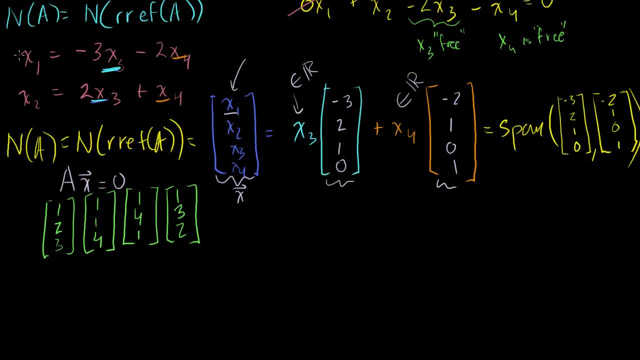 I could just write A as just this much of columns. But my question is: is this a linearly independent set? Linearly independent, And here you might immediately start thinking: well, when we said that something is linearly independent, so linearly independence. let me just write it like this: 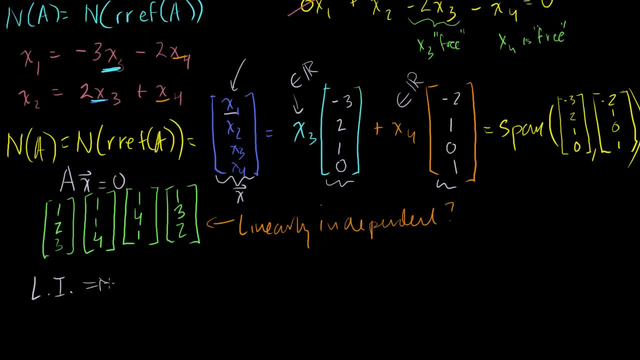 Linear independence implies that there's only one solution. we saw this, I think, two videos ago- that there's only one solution to Ax is equal to 0, and that is the 0 solution. that x is equal to the 0 vector. 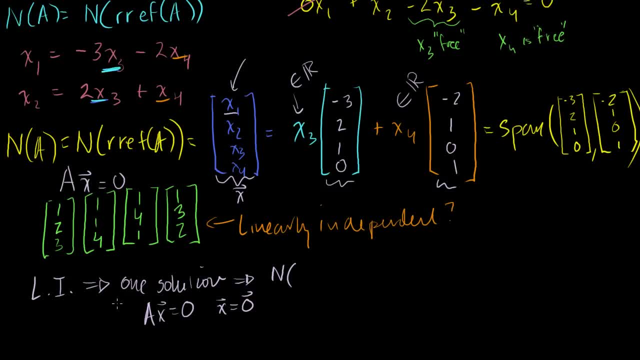 Or another way to say that is that the null space of my matrix A is equal to just the 0 vector. That's what linear independence implies, and it goes both ways. If my null space is just the 0 vector, then I know it's linearly independent. 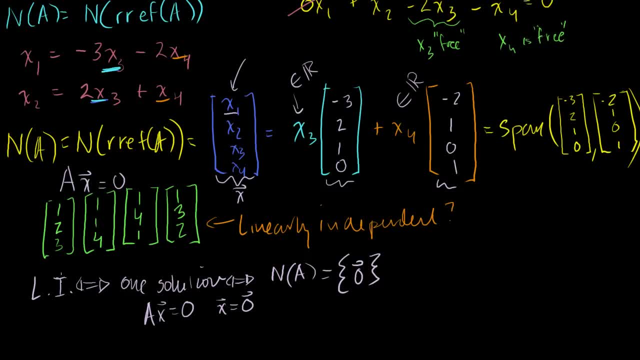 If my null space includes other vectors, then I'm not linearly independent. Now my null space of A: what does it include? Is it just the 0 vector? Well, no, it includes every linear combination of these guys. it includes an infinite number of vectors. 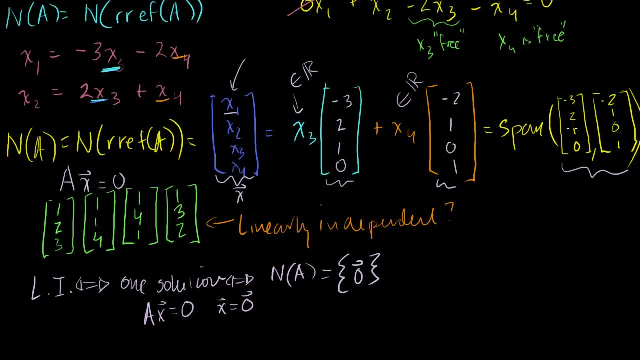 It's not just one solution. Obviously, 0 vector is contained here. if you just multiply both of these, if you pick 0 for that and that, it's contained. but you can get a whole set of vectors. So because the span of this guy, so you can kind of 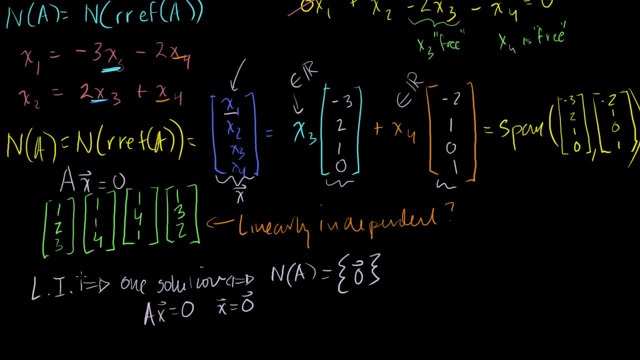 If my null space is just the 0 vector, then I know it's linearly independent. If my null space includes other vectors, then I'm not linearly independent. Now my null space of A: what does it include? Is it just the 0 vector? 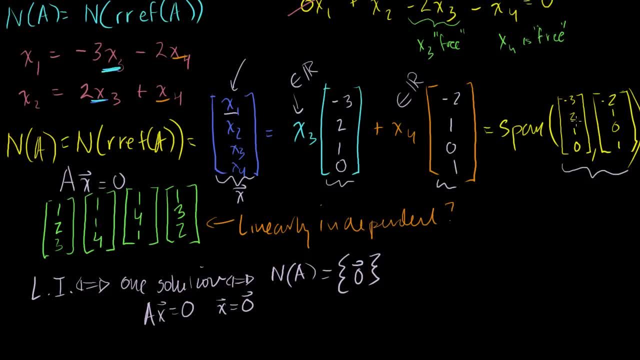 Well, no, It includes every linear combination of these guys. It includes actually an infinite number of vectors. It's not just one solution. Obviously, 0 vector is contained here, If you just multiply both of these, if you pick 0 for that. 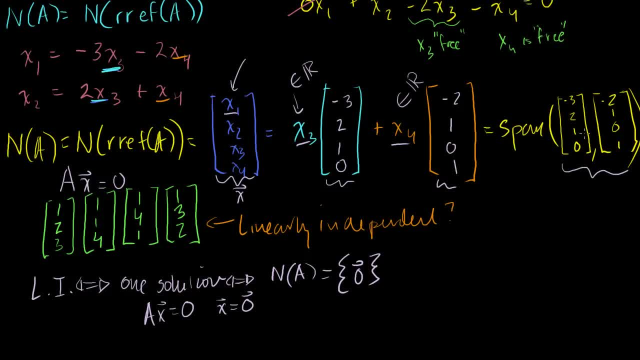 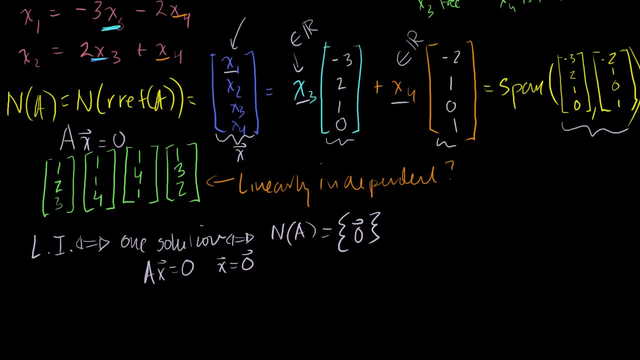 and that it's contained, But you can get a whole set of vectors. So because the span of this guy, so you can kind of, you know, the null span of A, the null space. sorry, the null space of A does not just contain the 0 vector. 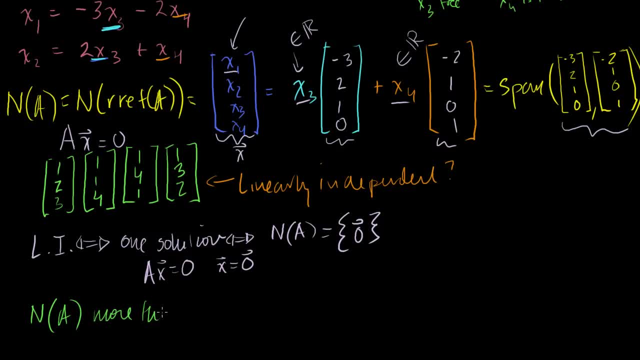 So it has more than just 0.. So what does that mean? Well, that means that there's more than one solution to this, And that means that this is a linearly dependent set. And what does that mean? Well, at the very beginning of the video, I said: what's the? 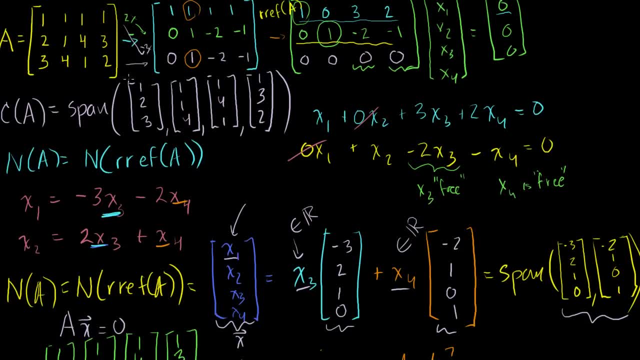 column space of A. And we said, oh, the column space of A is just the span of the column vectors, right? And I just wrote it out like that And I said, well, it's not clear whether this is a valid 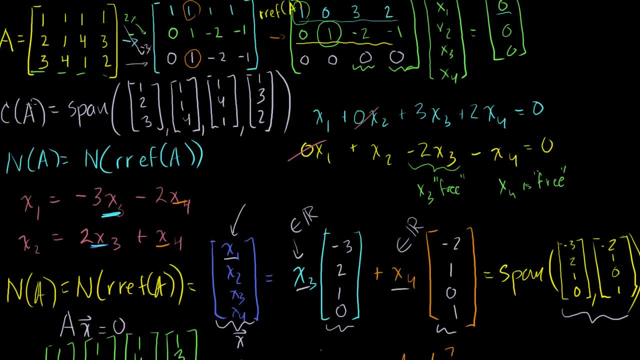 basis for the column space of A. And what's a basis? A basis is a set of vectors that span a subspace and they are also linearly independent, And we just showed that these guys are not linearly independent, not linearly independent. 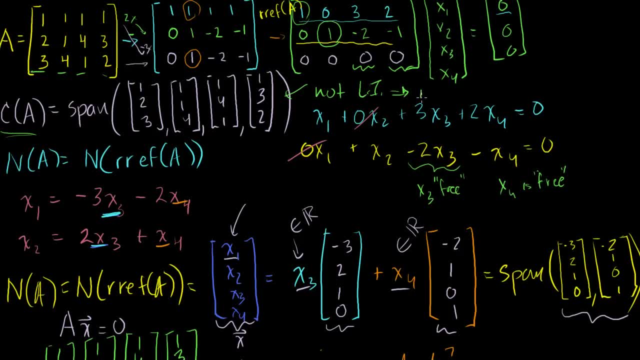 Right, Not linearly independent. So that means that they are not a basis for the column space of A. They do span the column space of A, by definition really, But they're not a basis They need to be linearly independent for. 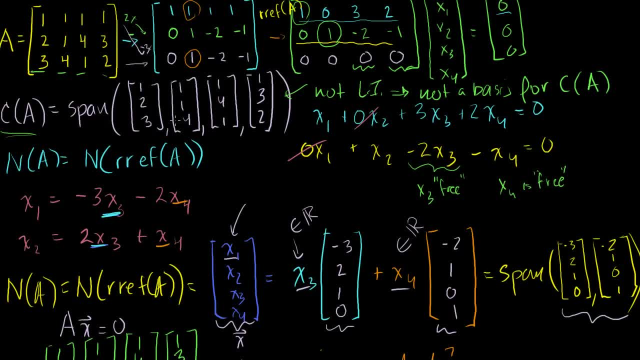 them to be a basis. So let's see if we can figure out what a basis for this column space would be, And to do that we just have to get rid of some redundant vectors. If I can show you that this guy can be represented by some, 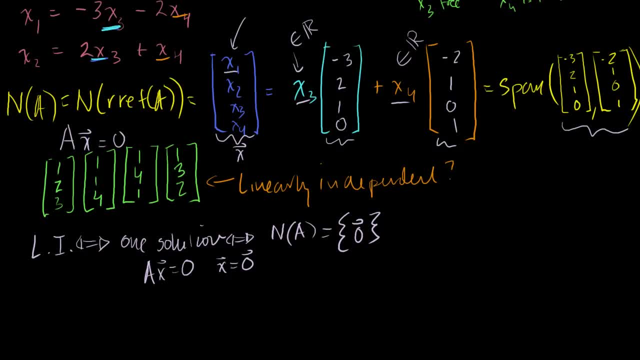 have the null span of A, the null space. sorry, the null space of A does not just contain the 0 vector, So it has more than just 0,. so what does that mean? Well, that means that there's more than one solution of this. 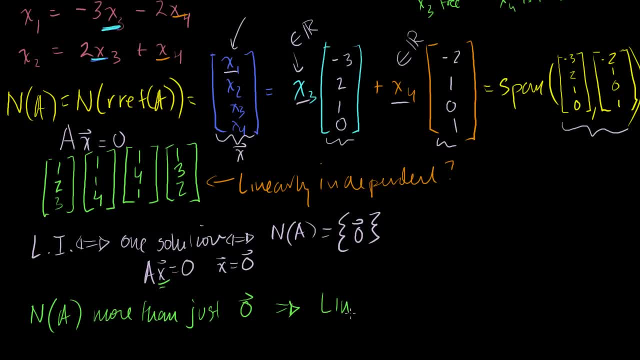 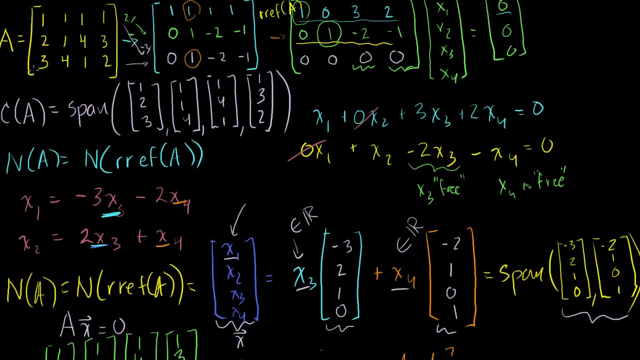 and that means that this is a linearly dependent set, Dependent set. And what does that mean? Well, at the very beginning of the video, I said: what's the column space of A? And we said, oh, the column space of A is just the span of. 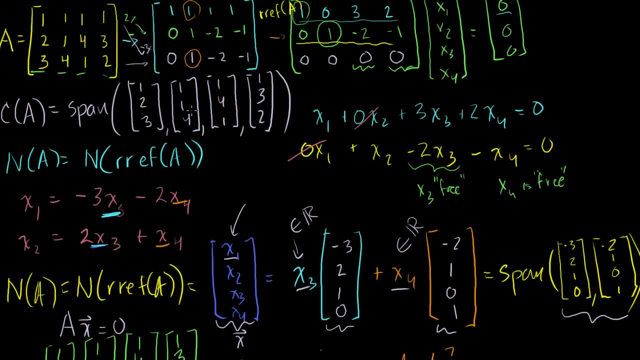 the column vectors, right? I just wrote it out like that And I said: well, it's not clear whether this is a valid basis for the column space of A, And what's a basis? A basis is a set of vectors that span a subspace and they 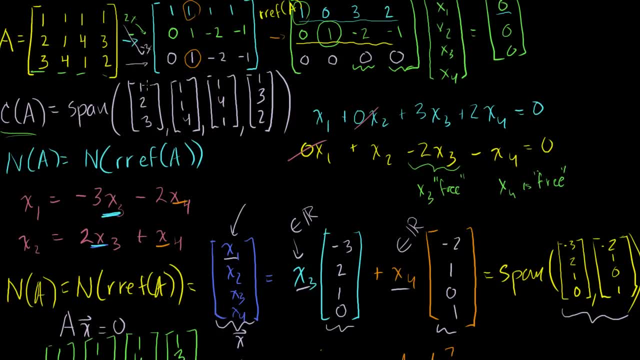 are also linearly independent. We just showed that these guys are not linearly independent, Not linearly independent, So that means that they are not a basis for the column space of A. They do span the column space of A by definition, really. 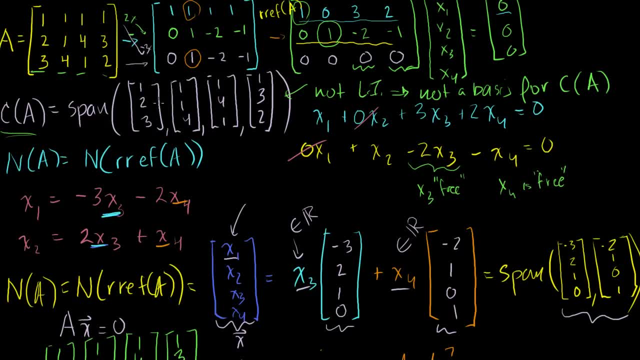 but they're not a basis. They need to be linearly independent for them to be a basis. So let's see if we can figure out what a basis for this column space would be, And to do that we just have to get rid of. 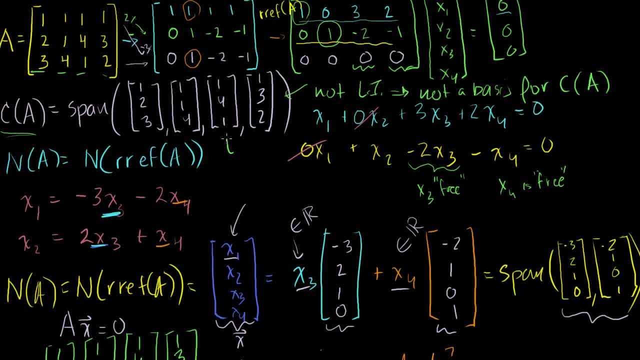 some redundant vectors. If I can show you that this guy can be represented by some combination of these two guys, then I can get rid of that guy. He's not adding any new information, Same with that guy Who knows? So let's see if we can figure this piece of the puzzle out. 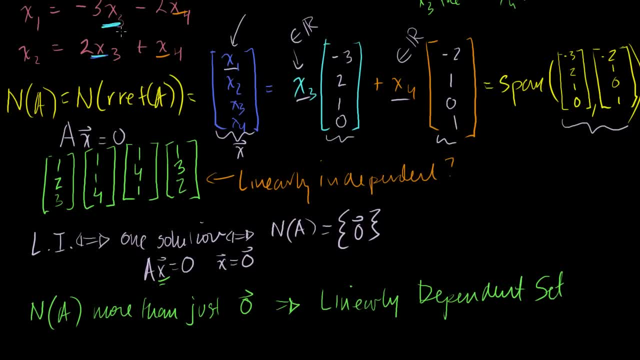 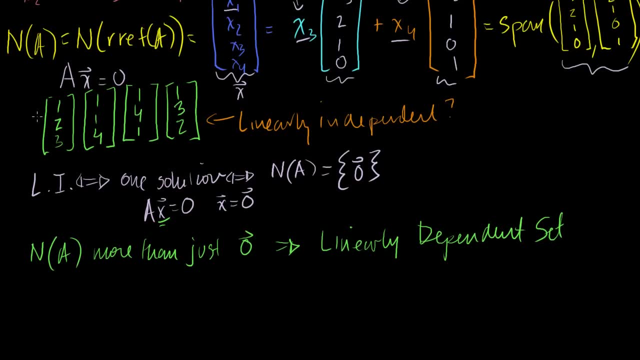 So we know already that x1, let me write it this way- that x1 times. maybe I'll just kind of leave you hanging and continue this in the next video, but we know that x1 times 1,, 2,, 3.. 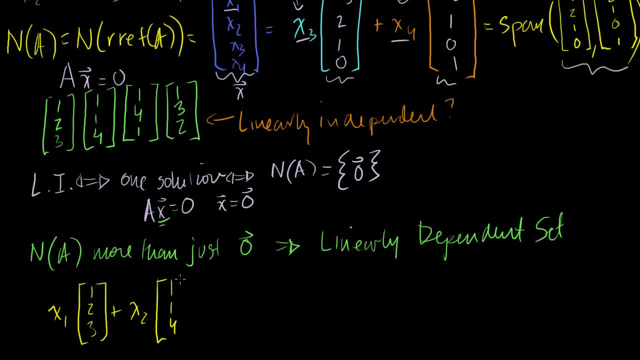 Plus x2 times 1, 1, 4.. Plus x3 times 1, 4, 1.. Plus x4 times 1, 3, 2. We know that this is equal to 0. Now, if we're able to solve for x4 in terms of, let's say, I: 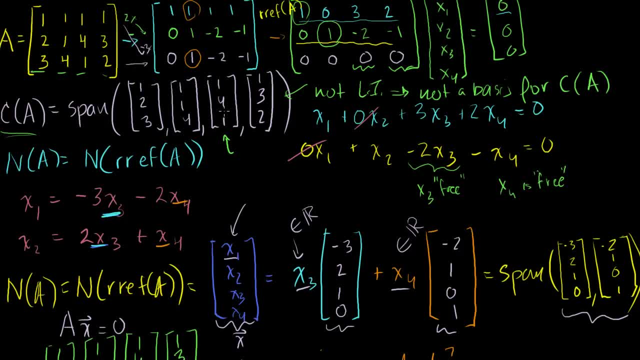 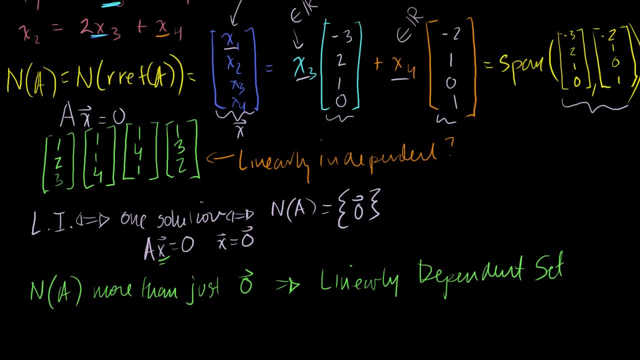 combination of these two guys, then I can get rid of that guy. He's not adding any new information, Same with that guy Who knows. So let's see if we can figure this piece of the puzzle out. So we know already that x1, let me write it this way- that 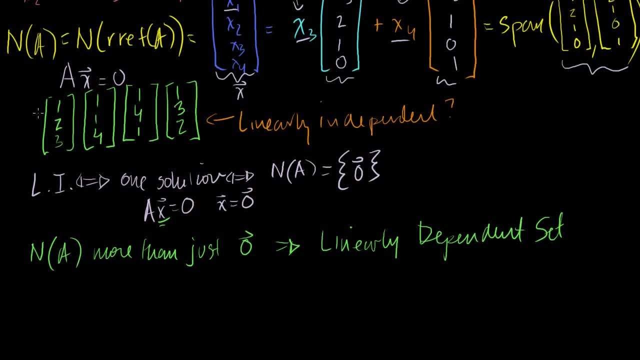 x1 times. maybe I'll just kind of leave you hanging and continue this in the next video, but we know that x1 times 1, 2, 3.. Plus x2 times 1, 1, 4.. Plus x3 times 1, 4, 1.. 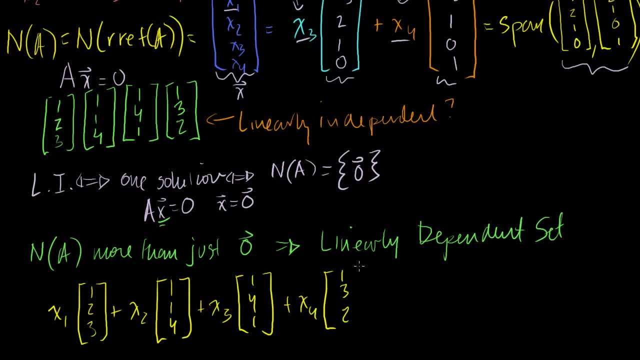 Plus x4 times 1,, 3, 2.. We know that this is equal to 0.. Now, if we're able to solve for x4 in terms of, let's say I can solve them in terms of. let me just think that I can. 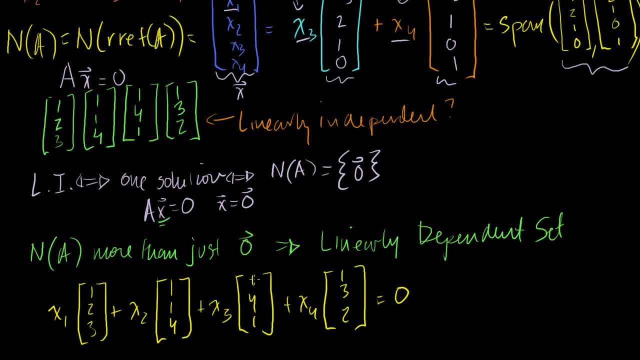 solve for the vectors that are associated with my free variables using the other vectors. Let me see if I can do that And you'll see it's actually pretty straightforward. So let's say, I want to figure out, I want to solve for x4.. 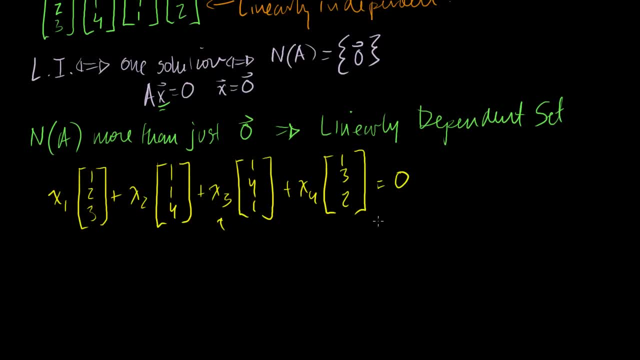 So if I subtract this from both sides of this equation, I get what I get minus. let me put it this way: Let me set x3 equal to 0. That was a free variable. I can do that. So if I set x3 is equal to 0, then what do I get here? 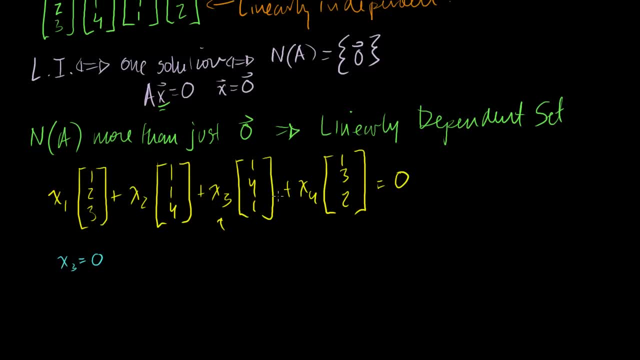 I get: if I set x3 equals 0, this guy disappears. And then if I subtract this from both sides of this equation, I get x1 times 1,, 2,, 3 plus x2 times 1, 1, 4 is 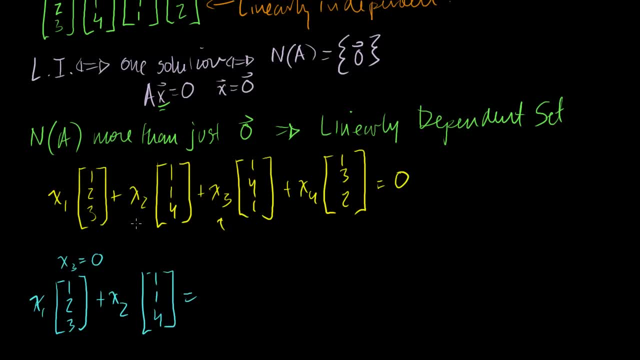 equal to. I'm just setting x3 equal to 0. That was a free variable, So I'm setting x3 equal to 0. So this whole thing disappears. So that is equal to minus x4 times 1,, 3,, 2.. 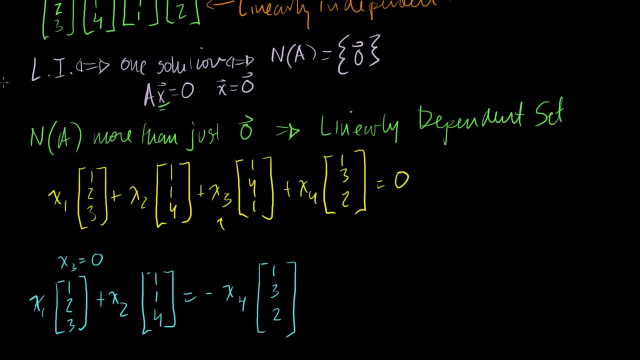 Let me set x1, sorry, let me set x4 to be equal to minus 1.. x4 is equal to minus 1.. If x4 is equal to minus 1, what is minus x4?? Well then, this thing will just be equal to 1.. 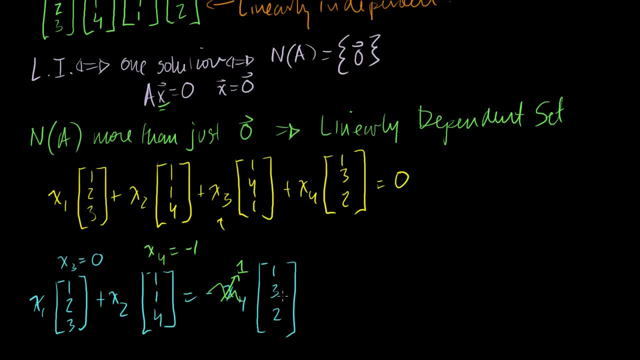 And I'll have x1 times 1,, 2, 3 plus x2 times 1, 1, 4 will equal this fourth vector right here. And can I always find things like this? Well, sure, I can actually find the particular ones. 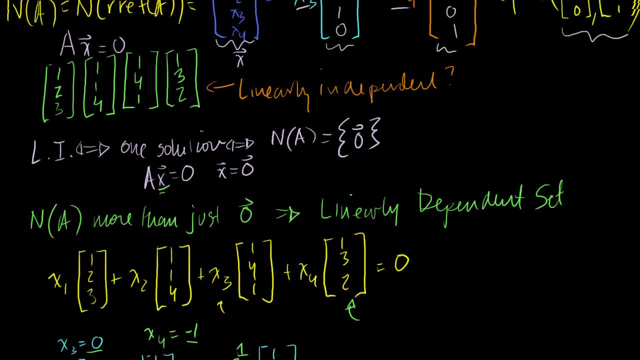 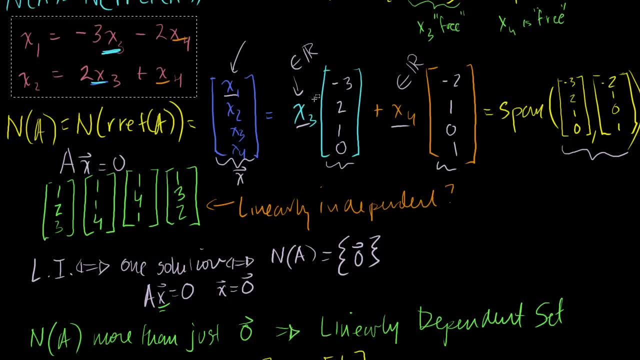 If x3 is equal to 0 and x4 is minus 1, let me copy and paste this So that I have up here. Let me copy and paste this. Sometimes it doesn't Edit, copy, edit, paste. There you go. 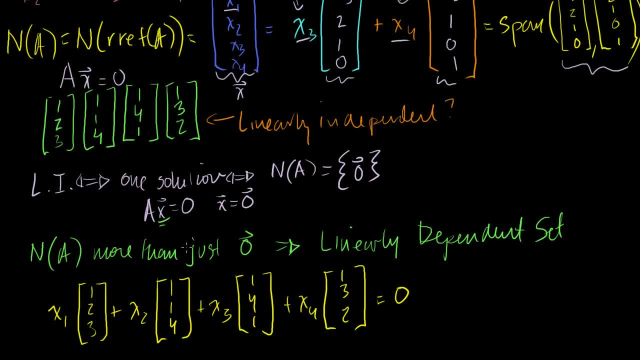 can solve them in terms of. let me just think that I can solve for the vectors that are associated with my free vectors, Free variables, using the other vectors. Let me see if I can do that And you'll see. it's actually pretty straightforward. 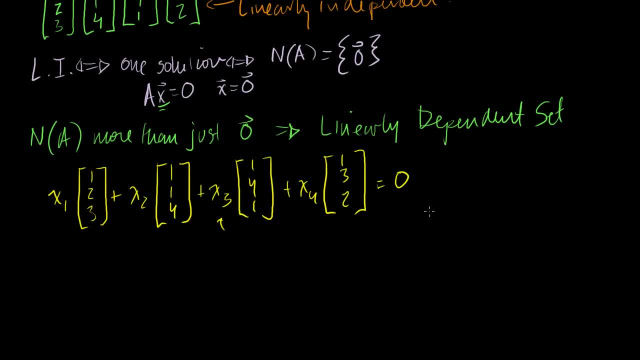 So let's say I want to figure out, I want to solve for x4.. So if I subtract this from both sides of this equation, I get what I get minus. let me put it this way: Let me set x3 equal to 0. 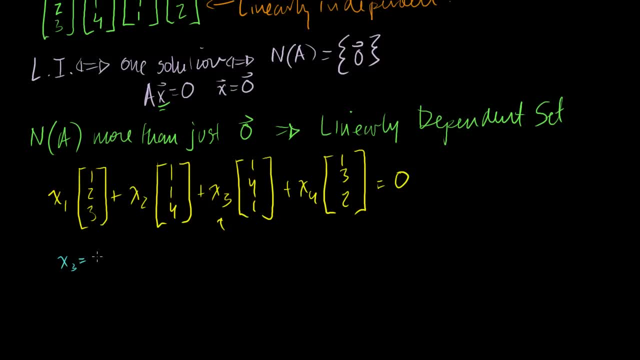 That was a free variable. I can do that. So if I set x3 is equal to 0, then what do I get here? If I set x3 equals 0, this guy disappears. And if I subtract this from both sides of this equation, I 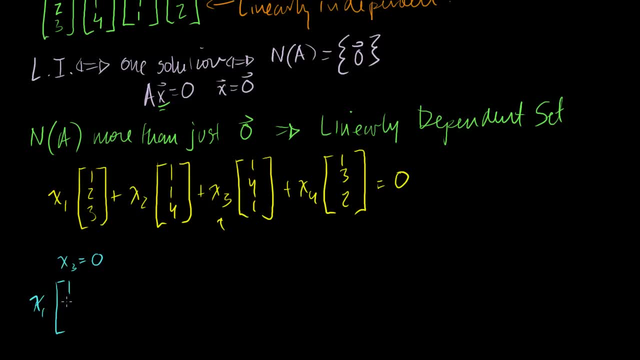 get x1 times 1,, 2,, 3 plus x2 times 1, 1, 4 is equal to. I'm just setting x3 equal to 0.. That was a free variable, So I'm setting x3 equal to 0, so this whole thing disappears. 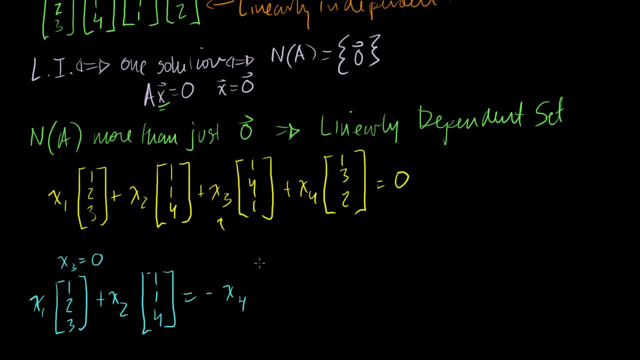 So that is equal to minus x4 over, or times 1,, 3, 2.. Now I set x3 equal to 0. Let me set x1, sorry, let me set x4 to be equal to minus 1.. 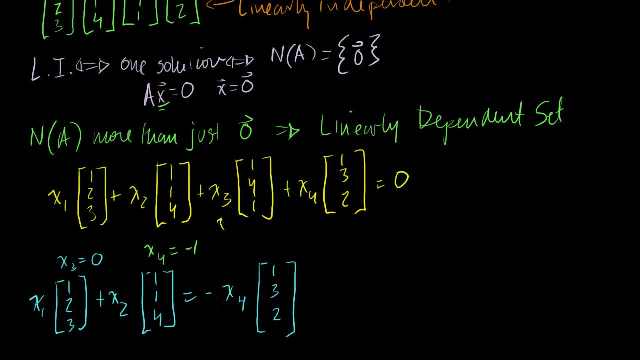 x4 is equal to minus 1.. If x4 is equal to minus 1, what is minus x4?? Well then, this thing will just be equal to 1. And I'll have x1 times 1,, 2, 3 plus x2 times 1, 1, 4 will. 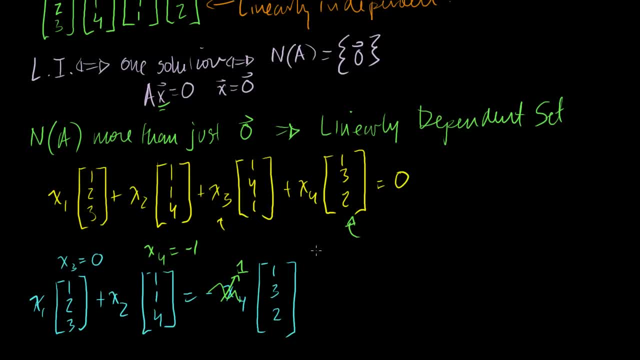 equal this fourth vector right here. And can I always find things like this? Well, sure, I can actually find the particular ones If x3 is equal to 0 and x4 is minus 1, let me copy and paste this over. 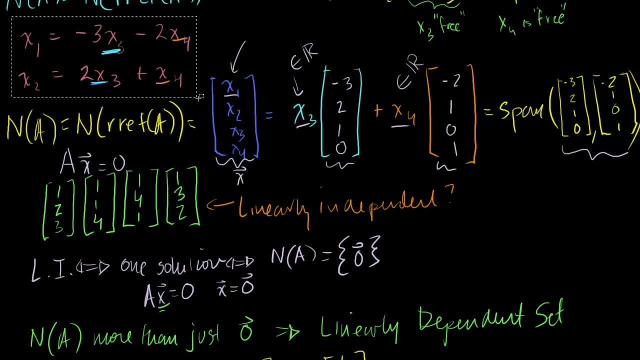 That I have up here. Let me copy and paste this. Sometimes it doesn't Edit, copy, edit paste. There you go. OK, let me scroll down a little bit. This is what we got when we figured out our null. 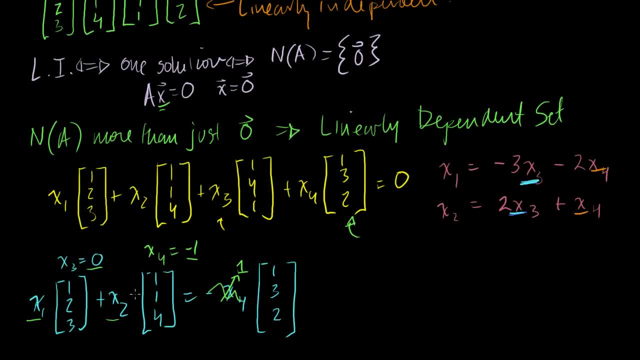 space right there. So if I'm setting- remember, these are the free variables- If I set x3 equal to 0 and x4 is equal to minus 1, what is x1?? Then this will imply that x1, well, it's equal to minus 3. 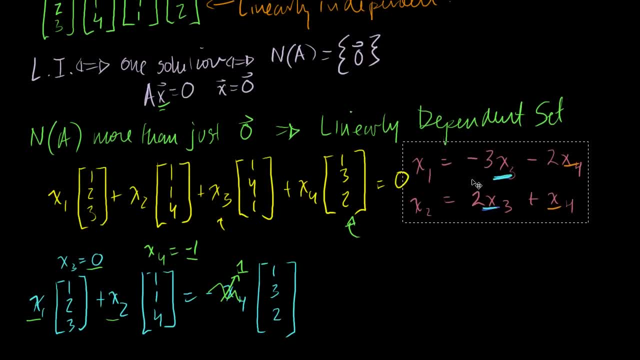 OK, let me scroll down a little bit. This is what we got when we figured out our null space right there. So if I'm setting, remember these are the free variables. If I set x3 equal to 0 and x4 is equal to minus 1.. 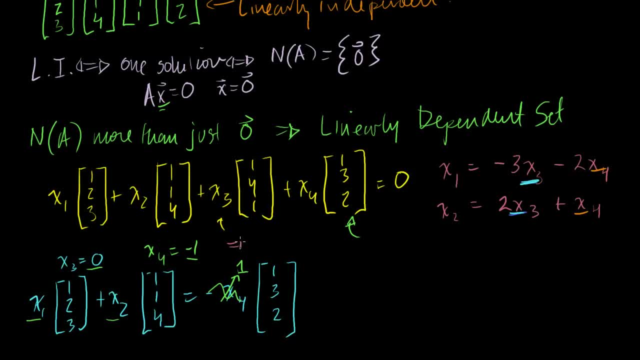 What is x1?? Then this will imply that x1, well, it's equal to minus 3 times x3. That's just 0. Minus 2 times x4. If x4 is minus 1, minus 2 times minus 1, x1 will equal 2.. 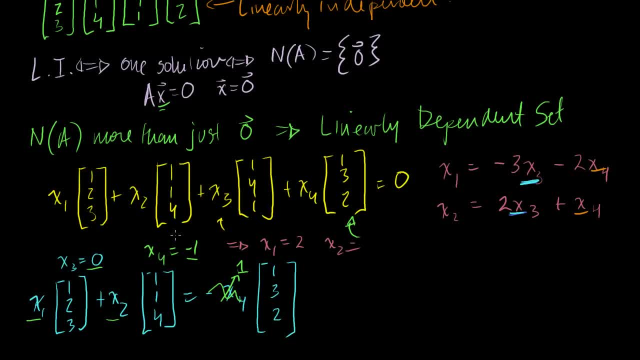 And then what will x2 be equal to? x2 is equal to 2 times x3, which is 0, plus x4. So it's equal to minus 1.. So I just showed you that if I set this equal to 2 and this 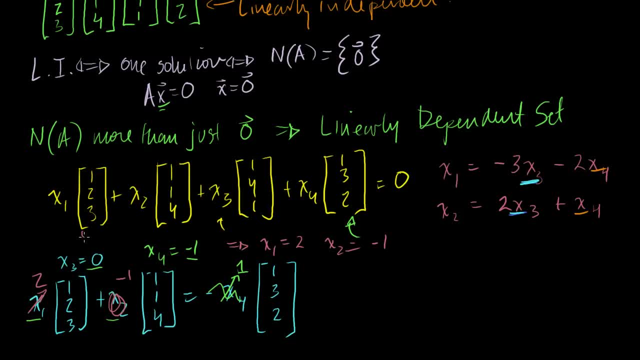 equal to minus 1.. I have a linear combination. I have a linear combination of this vector and this vector that can add up to this fourth vector, And you can even verify it: 2 times 1 minus 1 is equal to 1.. 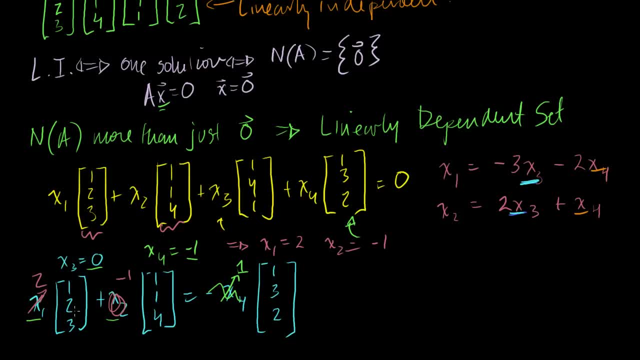 2 times 2 minus 1 is equal to 3.. 2 times 3 is 6.. Minus 4 is equal to 2.. So it checks out. So I just showed you using really our definitions, really looking at what were our free variables versus our. 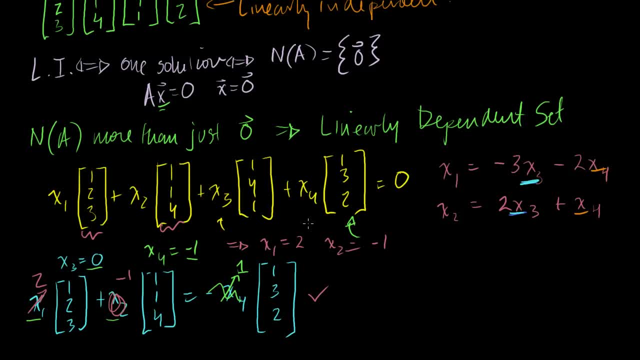 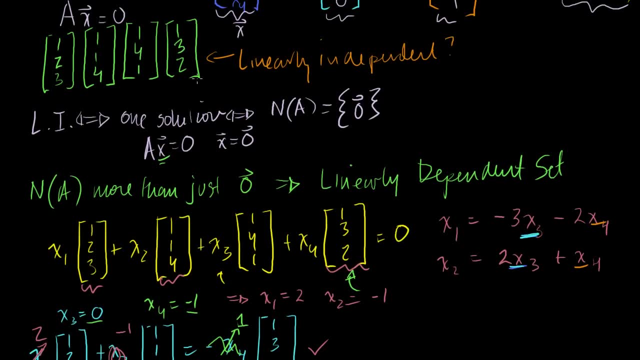 pivot variables. we were able to show you kind of just very simply solve for this third, This fourth vector, This fourth vector in terms of these first two. So we know, if we go back to the set, that this fourth vector is really unnecessary. 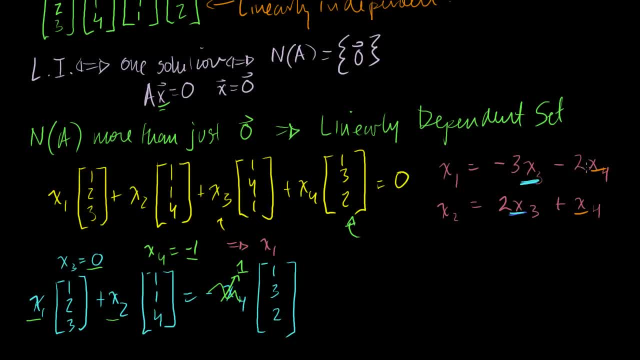 times x3, that's just 0, minus 2 times x4.. If x4 is minus 1, minus 2 times minus 1,, x1 will equal 2.. And then what will x2 be equal to? x2 is equal to 2 times x3, which is 0, plus x4.. 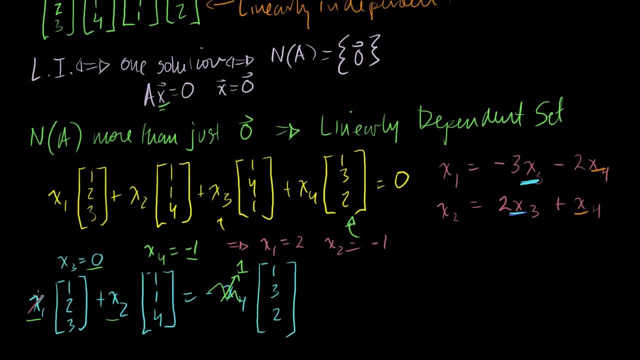 So it's equal to minus 1.. So I just showed you that if I set this equal to 2 and this equal to minus 1, I have a linear combination Of this vector and this vector that can add up to this fourth vector. 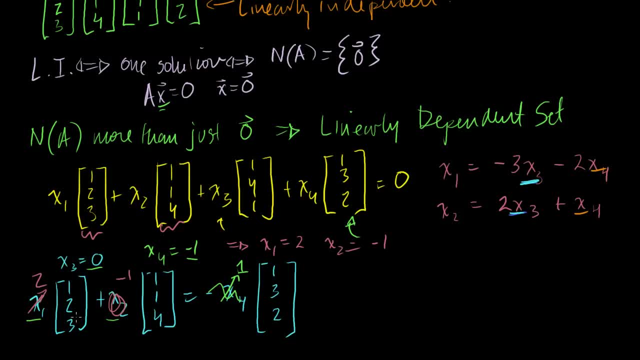 And you can even verify it: 2 times 1 minus 1 is equal to 1.. 2 times 2 minus 1 is equal to 3.. 2 times 3 is 6.. Minus 4 is equal to 2.. 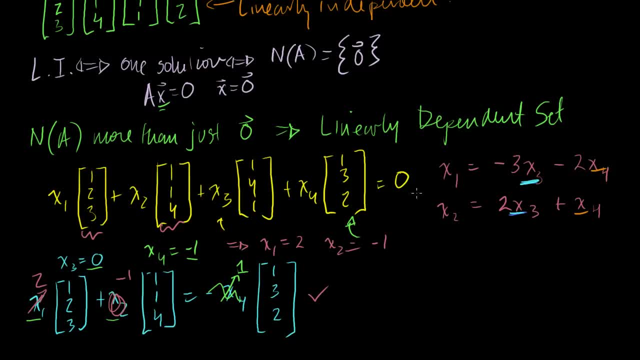 So it checks out. So I just showed you, using really our definitions, really looking at what were our free variables versus our pivot variables, we were able to show you kind of just very simply solved for this third, this fourth vector in. 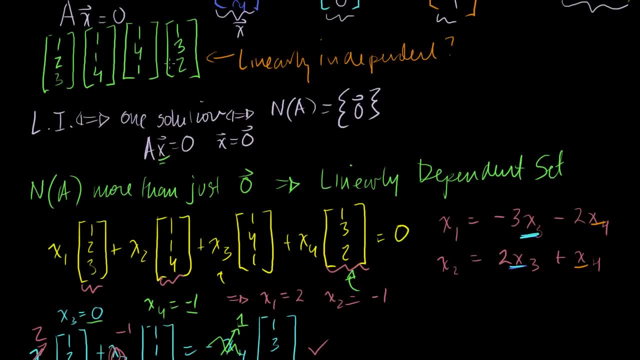 terms of these first two. So we know, if we go back to the set, that this fourth vector is really unnecessary, Really not adding anything to, I guess, the span of this set of vectors, because this guy can be written as a. 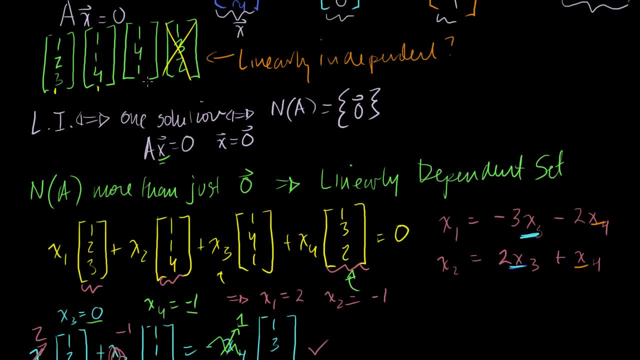 combination of this guy and this guy. Now let's see if this guy, if this third guy, we can do the same exercise. This is also dictated by a free variable, So let's see if I can write him as a combination of these. 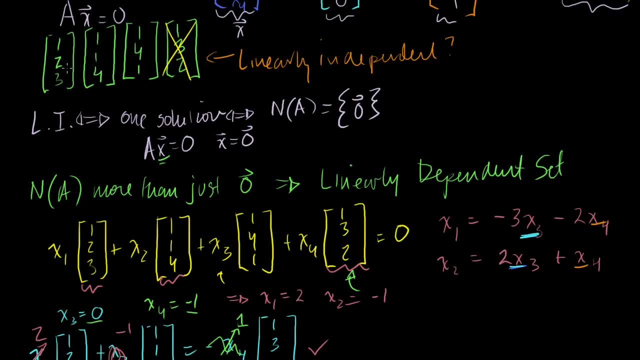 Really not adding anything to, I guess, the span of this set of vectors, Because this guy can be written as a combination of this guy and this guy. Now let's see if this guy, this third guy, we can do the same exercise. 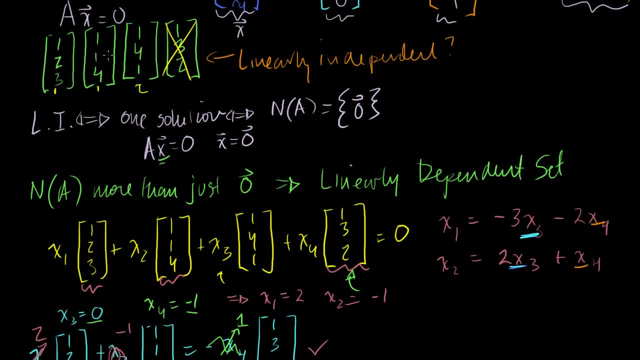 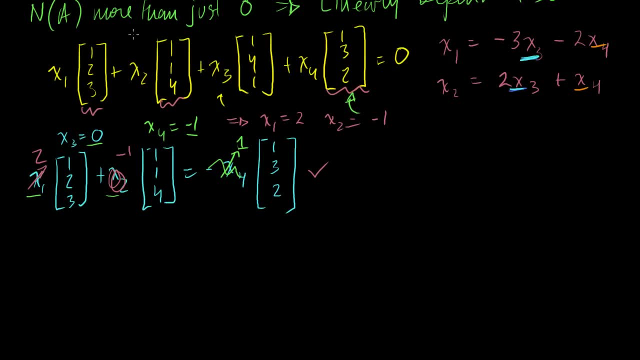 This is also dictated by a free variable, So let's see if I can write him as a combination of these first two. Well, we'll do the exact same thing. Instead of setting x3 equal to 0.. x3 equal to 0 and x4 equal to minus one, let's set x4. 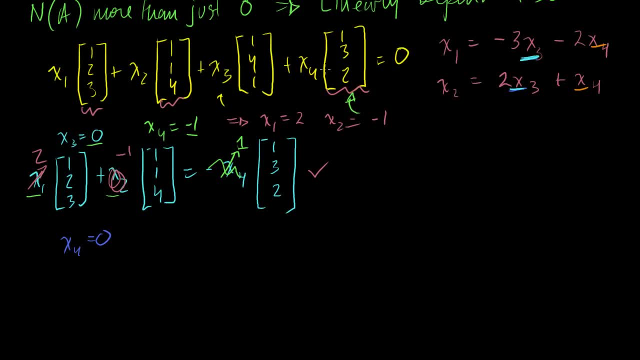 is equal to 0.. x4 is equal to 0. Because I want to cross that out. And let me set: x3 is equal to minus 1.. If x3 is equal to minus 1, so this equals minus 1, what is? 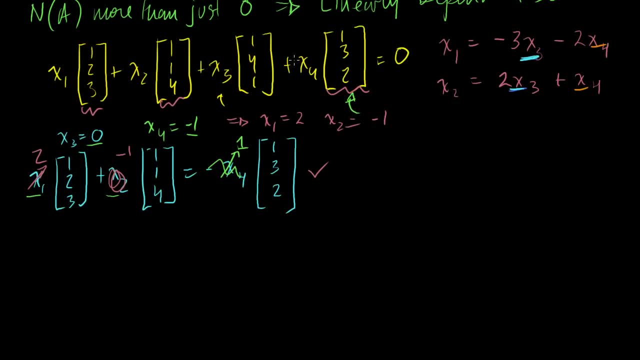 first two. Well, we'll do the exact same thing. Instead of setting x3 equal to 0 and x2 equal to 0,, we're going to set x4 equal to minus 1.. Let's set. let us set x4 is equal to 0, because I want to. 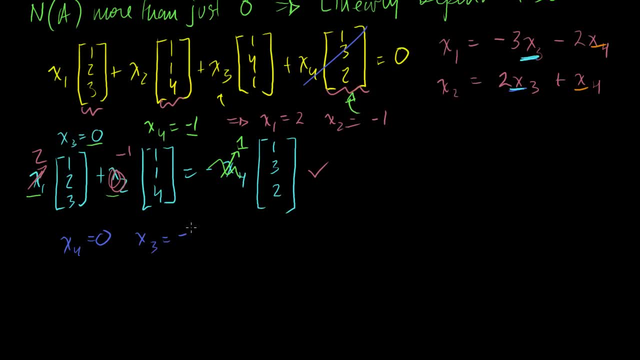 cross that out And let me set: x3 is equal to minus 1.. If x3 is equal to minus 1, so this equals minus 1, what is this equation reduced to? We get x1 times 1,, 2, 3.. 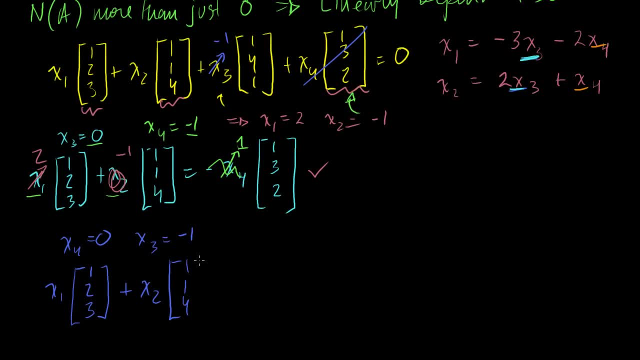 Plus x2 times 1, 1, 4.. If this is minus 1 times 1, 4, 1, and then we add it to both sides of this equation, we get plus 1 times 1, 4, 1.. 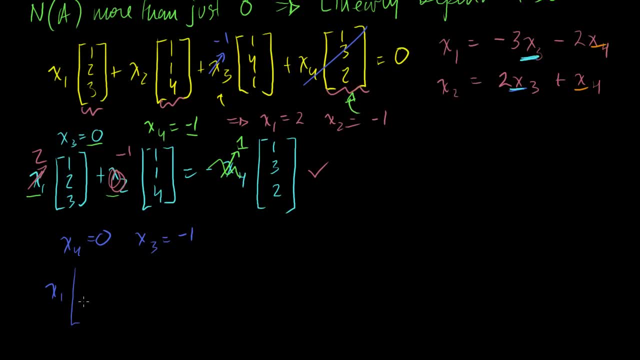 this equation reduced to, We get x1 times 1, 2, 3.. Plus x2 times 1, 2, 3.. 1, 1, 4 is equal to: if this is minus 1 times 1, 4,, 1, and. 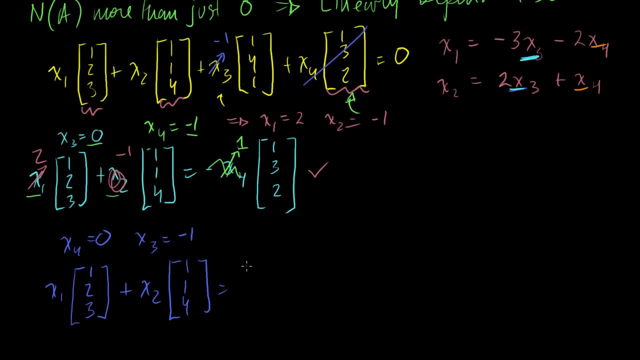 then we add it to both sides of this equation, we get plus 1 times 1,, 4,, 1.. And once again we can just solve for our x1's and x2.. If x4 is 0 and x3 is minus 1, then x1, x4 is 0,, so x3 is. 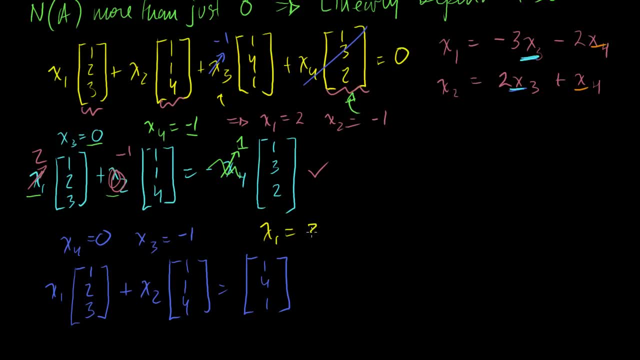 just minus 3 times x3.. So x1 would be equal to 3, right, Minus 3 times minus 1.. And what would x2 be equal to? x4 is 0, we can ignore that. x2 would be equal to minus 2.. 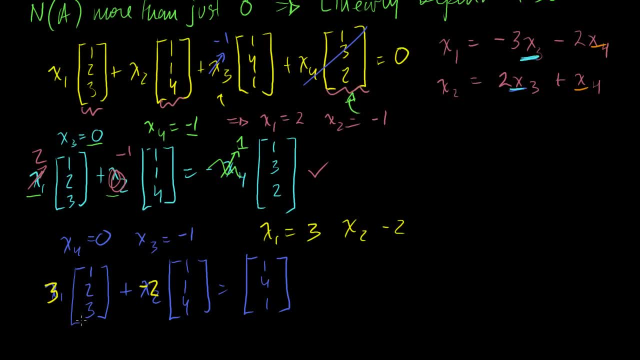 So this would be 3, and then this would be minus 2.. Let's see if it works out. 3 times 1 minus 2 is 1.. 3 times 2 minus 2 is 4.. 3 times 3 minus 8 is 1.. 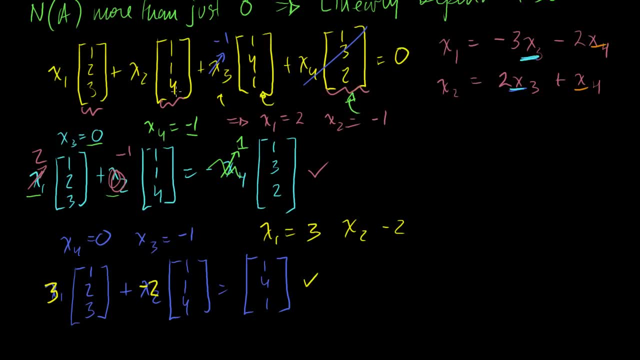 It checks out. So I'm able to write this vector that was associated with a free variable as a linear combination of these two, So we can get rid of him from our set. So now I've shown that this guy can be written as a linear. 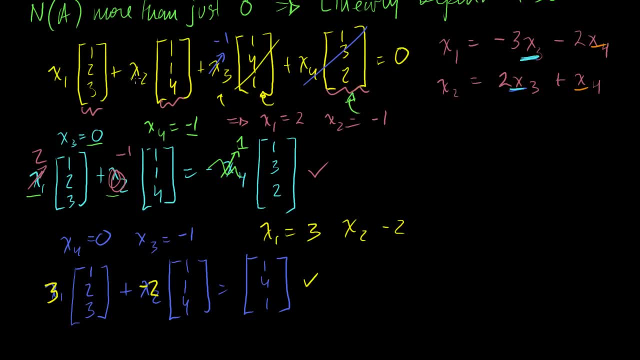 combination of these two. This guy can be written as a linear combination of these two, So the span of all of those guys should be equal to the span. so let me write it this way. The column space of A I can now rewrite. 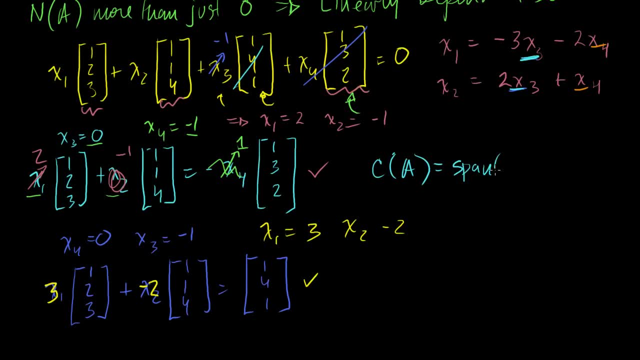 It was before. it was the span of all of those vectors. It was the span of all of the column vectors: v1,, v2,, v3, and v4.. Now I just showed you that v3 and v4 can be rewritten in. 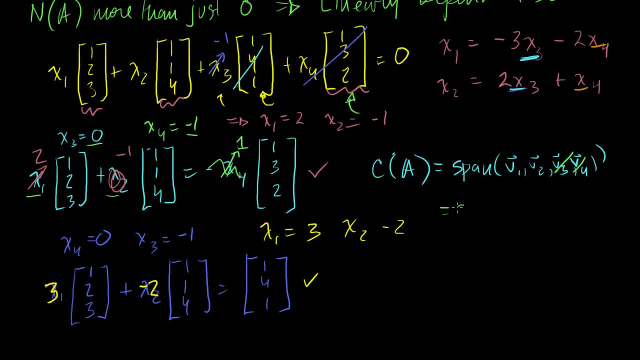 terms of v1 and v2.. So they're redundant. So that is equal to the span of v1 and v2, which are just those two vectors: Vector 1, 2, 3, and vector 1, 1, 4.. 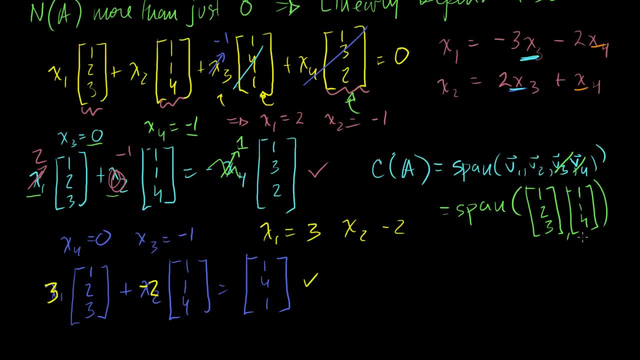 Now, are any of these guys redundant? Can I express one of them as a linear combination of the other? And essentially, when I'm talking about the linear combination of only one other vector, it's just multiplying it by a scalar. Well, let's think about that. 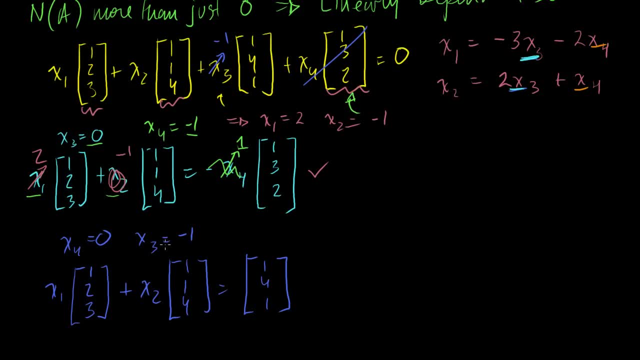 And once again we can just solve for our x1's and x2.. If x4 is 0 and x3 is minus 1, then x1, x4 is 0, so x3 is just minus 3 times x3. 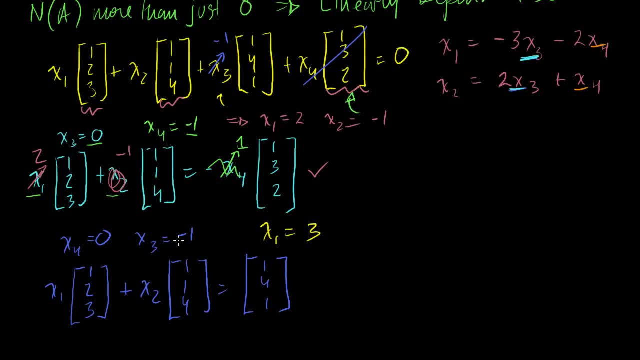 So x1 would be equal to 3, right, Minus 3 times minus 1.. And what would x2 be equal to? x4 is 0. We can ignore that. x2 would be equal to minus 1.. 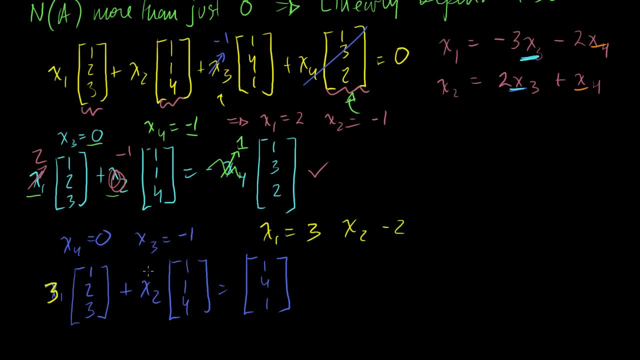 x2 would be equal to minus 1.. x2 would be equal to minus 1.. x2 would be equal to minus 2.. So this would be 3, and then this would be minus 2.. Let's see if it works out. 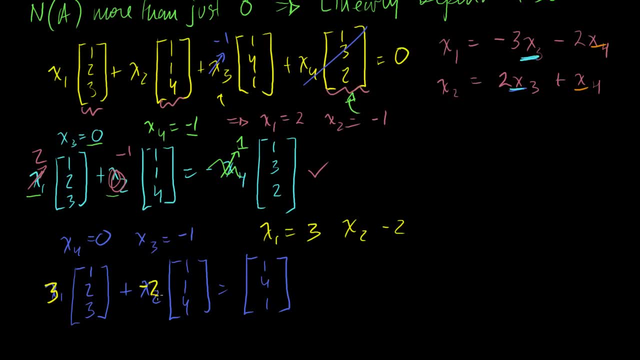 3 times 1 minus 2 is 1.. 3 times 2 minus 2 is 4.. 3 times 3 minus 8 is 1.. It checks out So I'm able to write this vector that was associated. 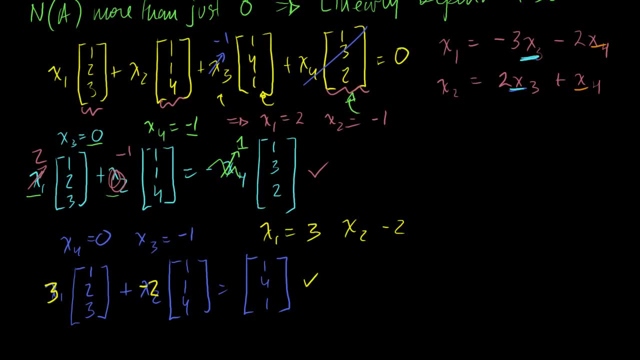 with a free variable as a linear combination of these two, so we can get rid of him from our set. So now I've shown that this guy can be written as a linear combination of these two. This guy can be written as a linear combination of these: 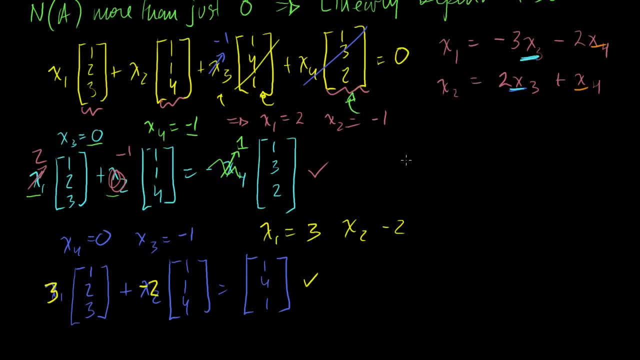 two, The span of all of those guys should be equal to the span. So let me write it this way: The column space of A- I can now rewrite. It was before. it was the span of all of those vectors. It was the span of all of the column vectors v1,, v2,, v3,. 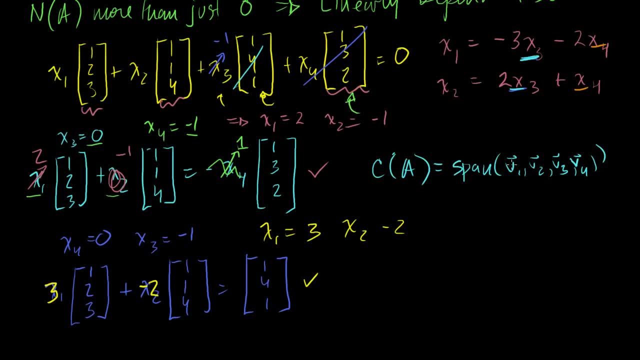 and v4.. Now I just showed you that v3 and v4 can be rewritten in terms of v1 and v2, so they're redundant. So that is equal to 1. The span of v1 and v2, which are just those two vectors. 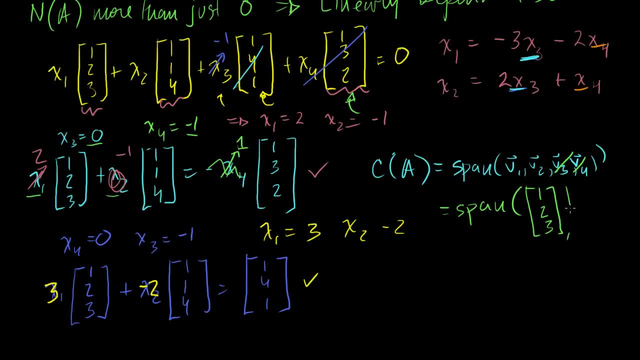 1, vector 1, 2, 3, and vector 1, 1, 4.. Now, are any of these guys redundant? Can I express one of them as a linear combination of the other? And essentially, when I'm talking about the linear? 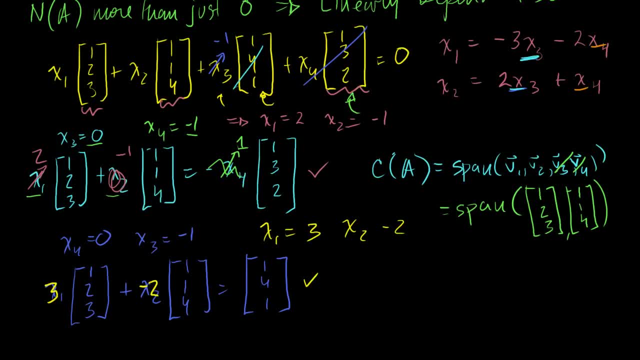 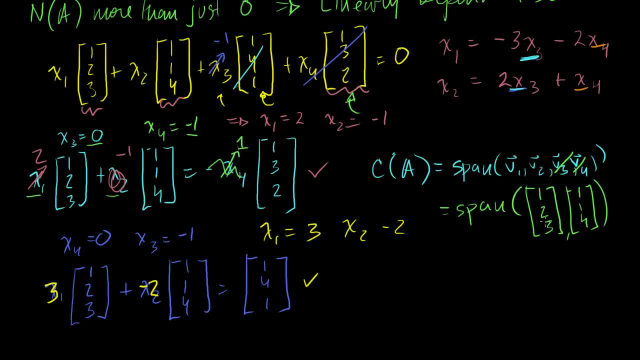 entry to that entry. I'm just multiplying by 1.. But if I multiply this whole vector times 1, then I'm going to get a 2 here and I'm going to get a 3 here, So it won't work. 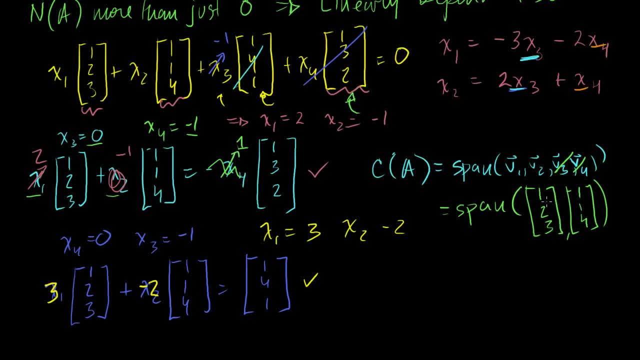 There's multiple ways you can show this, But the easiest way is: well, look to go from this entry to that entry. I'm just multiplying by 1.. But if I multiply this whole vector times 1, then I'm going to get a 2 here and I'm going to get a 3 here. 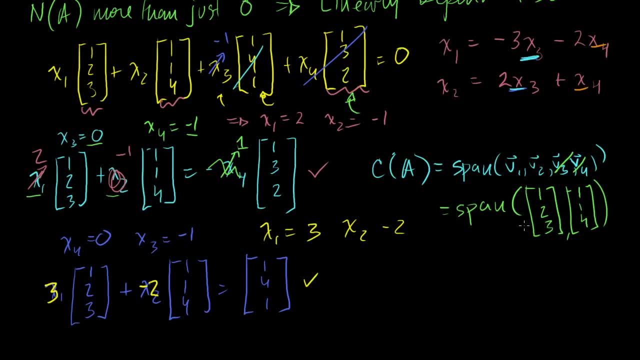 So it won't work. Let me put it this way If I want to represent this guy as a scalar multiple of that guy. So any scalar multiple of 1,, 2, 3 is going to be equal to 1c. 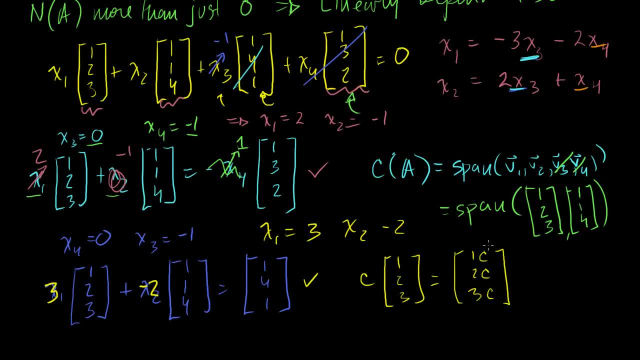 2c, 3c, Right. And so we're saying this guy has to be represented somehow. like that, If we say that this guy is somehow a scalar, it somehow can be represented by that guy. So that would have to be equal to 1, 1, 4.. 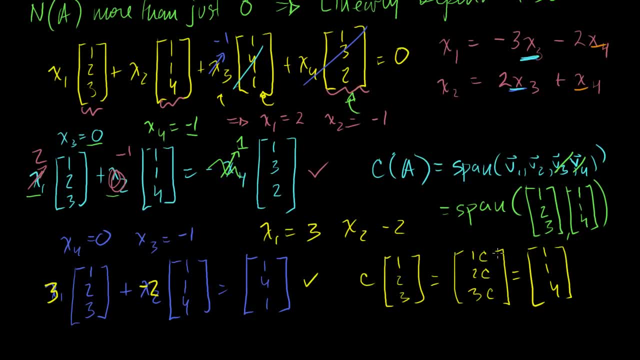 When you look at this top entry, it implies that c would have to be equal to 1.. When you just, c is equal to 1.. But when you look at this second entry, you think that c would have to be equal to 1 half. 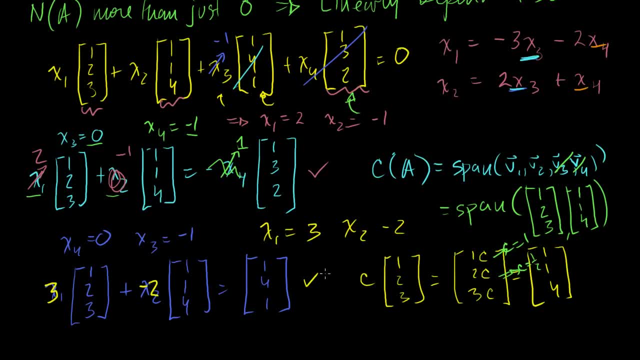 So you get a contradiction Over here. c would have to be equal to 4 thirds, So there's no c where this will work. There's no multiple of c, And you can work that both ways. So there's no way that you can represent one of these guys as. 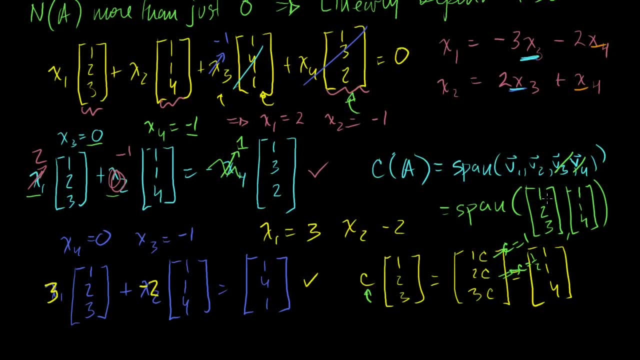 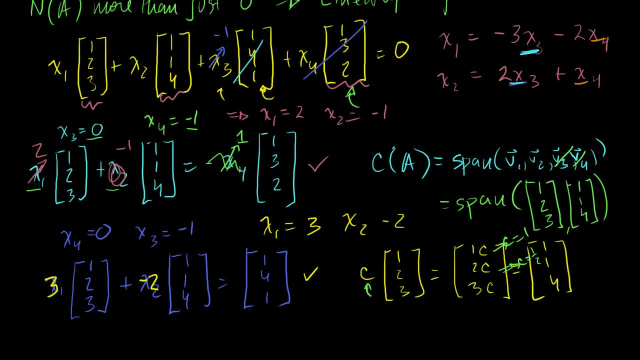 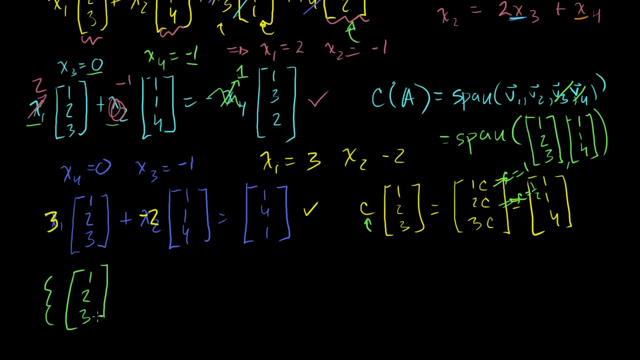 a linear combination of the other And you can actually prove other ways, maybe more formally, that this is linearly independent. But given that this is linearly independent, I think you're satisfied with that. We can then say that the set of vectors 1, 2, 3, and 1, 1,. 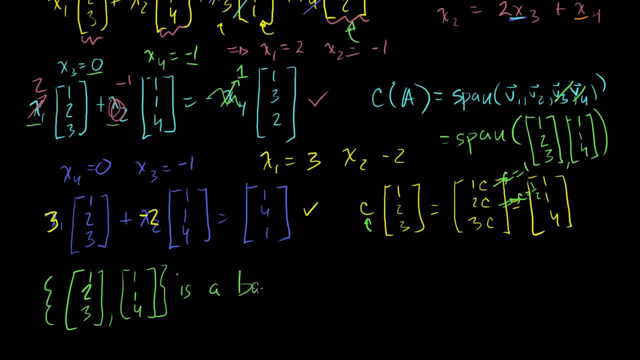 4,. this is a basis for the column span of A. Now I'm going to let you go in this video because I think I've gone well over time, But what I'm going to do in the next few videos is now that. 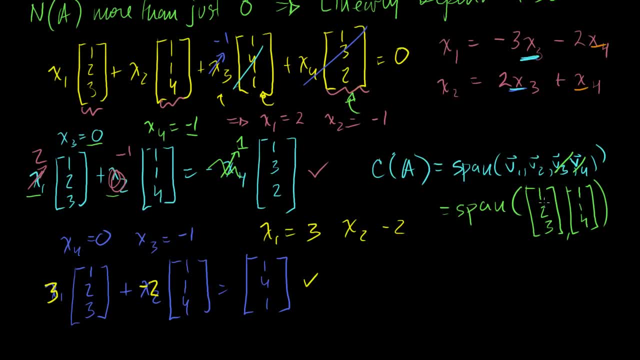 Let me put it this way: If I want to represent this guy as a scalar multiple of that guy, So any scalar multiple of 1,, 2,, 3 is going to be equal to 1c, 2c, 3c, right. 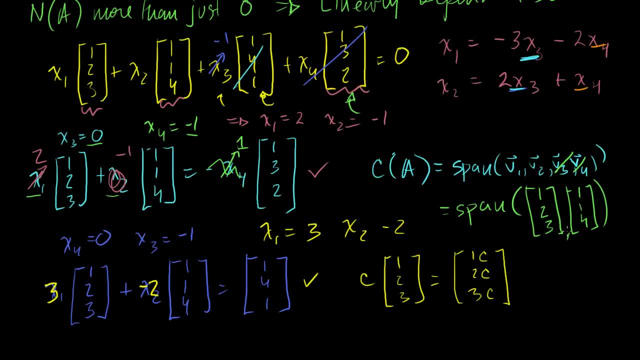 And so we're saying this guy has to be represented somehow. like that, If we say that this guy is somehow a scalar is somehow going to be represented by that guy. So that would have to be equal to 1, 1, 4.. 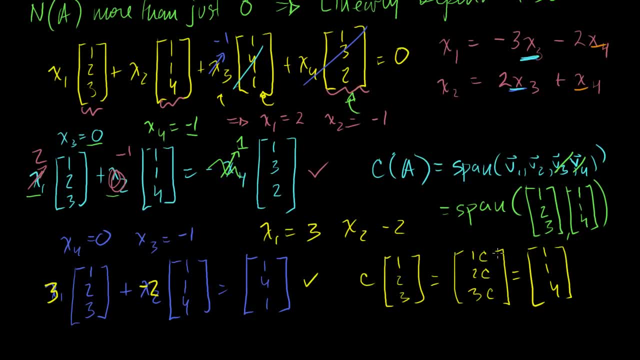 When you look at this top entry, it implies that c would have to be equal to 1.. When you just, c is equal to 1.. But when you look at this second entry, you think that c would have to be equal to 1 half. 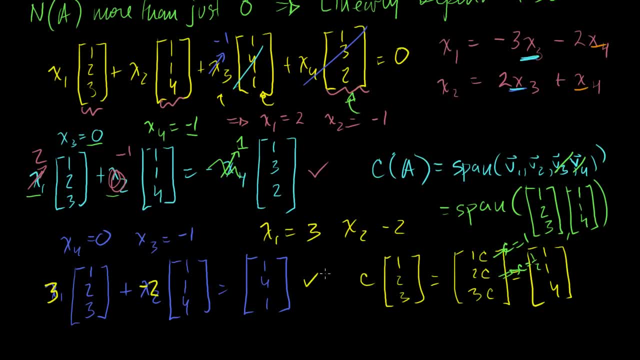 So you get a contradiction Over here. c would have to be equal to 4 thirds, So there's no c where this will work. There's no multiple of c, And you can work that both ways. So there's no way that you can represent one of these. 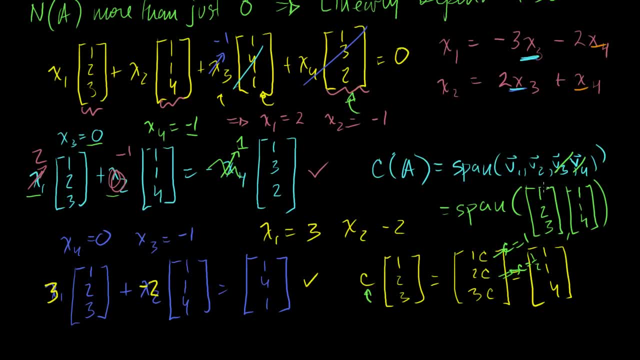 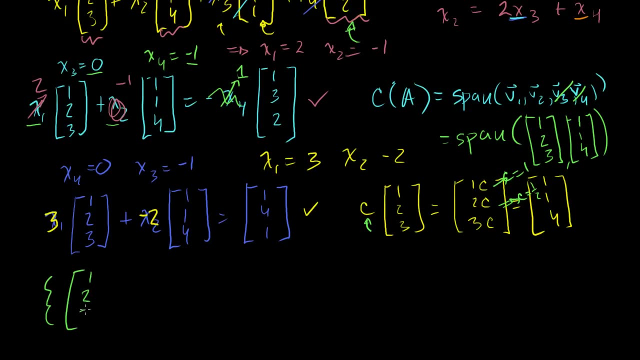 guys as a linear combination of the other And you can actually prove other ways, maybe more formally, that this is linearly independent. But given that this is linearly independent, I think you're satisfied with that. We can then say that the set of vectors 1, 2, 3, and 1, 1,. 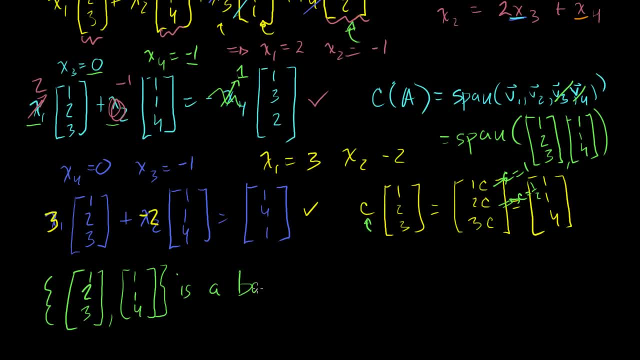 4,. this is a basis. This is a basis for the column span of A. Now I'm going to let you go in this video because I think I've gone well over time, But what I'm going to do in the next few videos is now that. 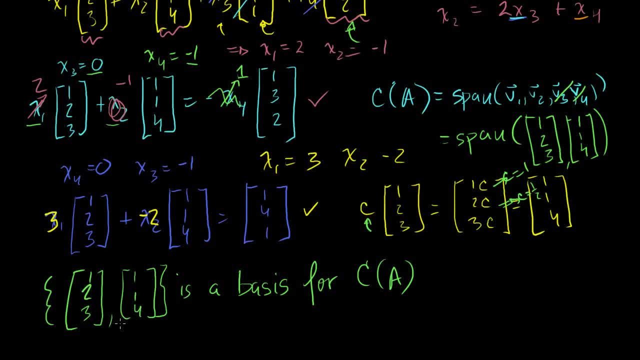 I've established that this is a basis for the column span of A. we can attempt to visualize it, Because we can say that the column span of A is equal to the span of these two vectors And we can think about what the span of those two vectors are. 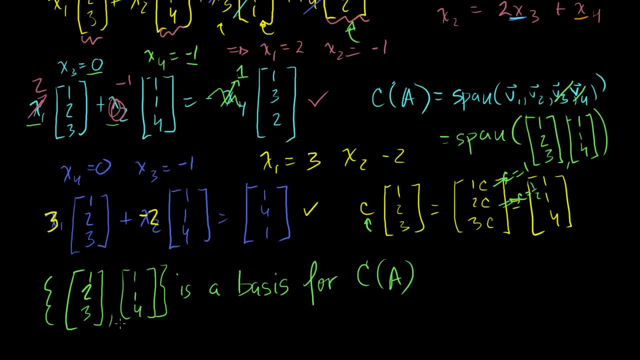 I've established that this is a basis for the column span of A. we can attempt to visualize it, Because we can say that the column span of A is equal to the span of these two vectors And we can think about what the span of those two vectors are. 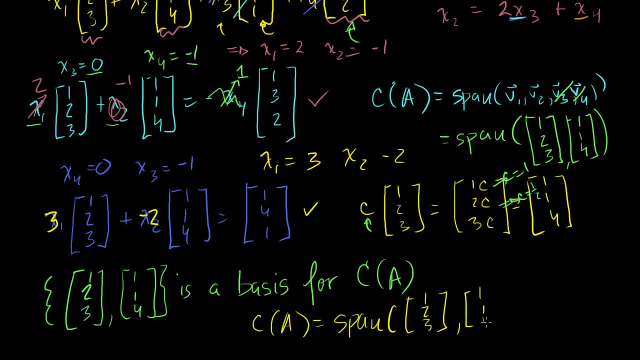 We're going to see that it's a plane in R3. Span of 1, 1, 4.. And just as a quick reminder, I said it a couple of times, When I say it's a basis, all I'm saying is that these guys